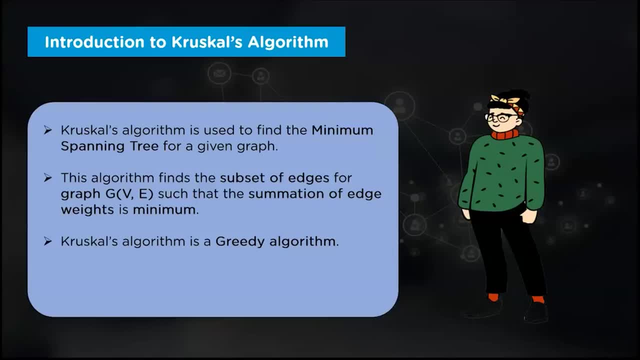 given age does not form a cycle. Also, it picks the age with minimum cost at first and the age with maximum cost at last. Hence we can say that the Kruskal's algorithm makes sense by using this data structure to find global optimal solutions. That is why it. 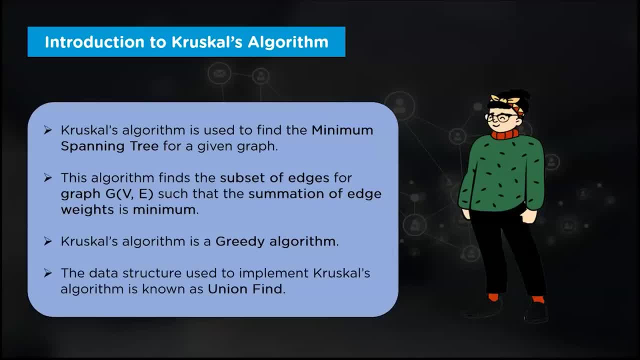 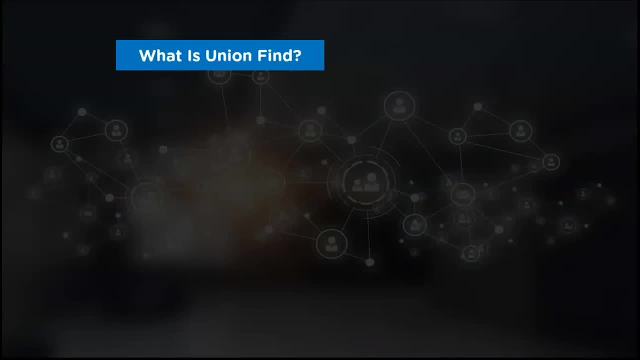 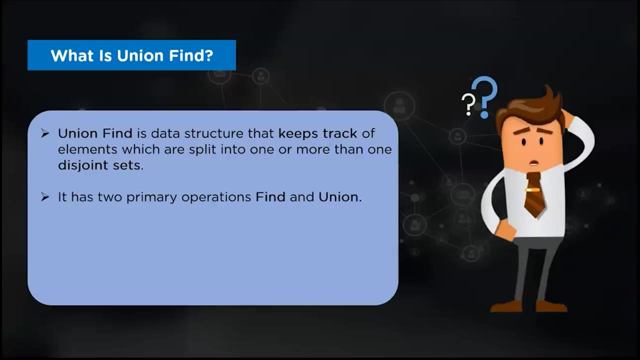 is also considered as a greedy algorithm. The data structure that we are going to use for implementing this Kruskal's algorithm is union fine. But now you must be thinking what exactly is this union fine data structure and how it works. Well, union fine is a data. 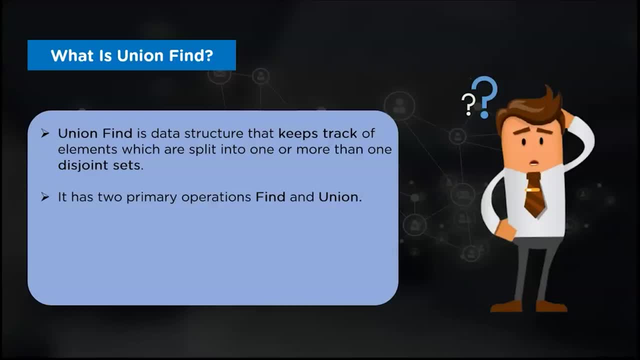 structure that keeps stacks of elements that are split into one or more than one disjoint sets. A set is a collection of two distinct groups or clusters that do not have a single common element. The union fine features two important operations named as find and union The operation. 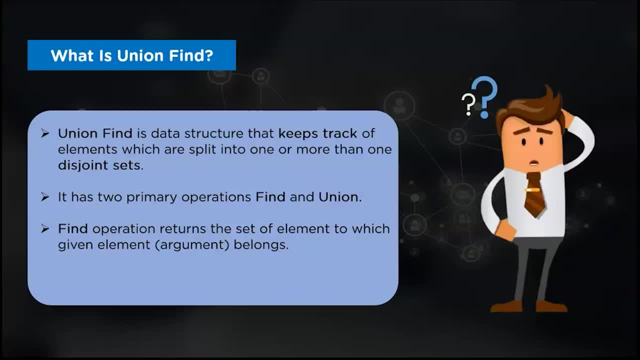 find returns the set or group to which the provided element belongs. Basically, it constructs a bisection between the object provided and its set, Whereas the union function joins two distinct disjoint sets to create a single subset. Let's understand how this data structure works with the help of real life example. 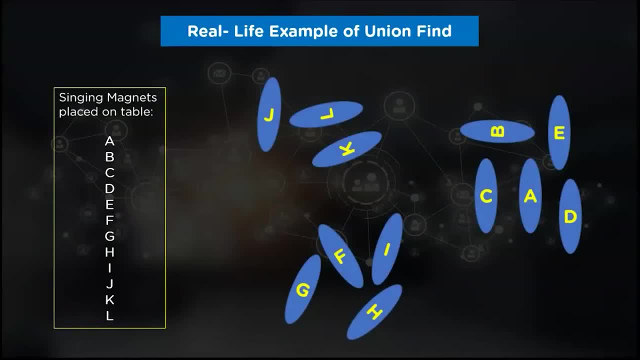 Let's say we have some sinking magnets placed on table with a higher magnetic affinity towards each other. All these sinking magnets present on the table are color coded with sky blue color. Now, due to the high magnetic attraction, the magnets A to E will form a strong magnetic 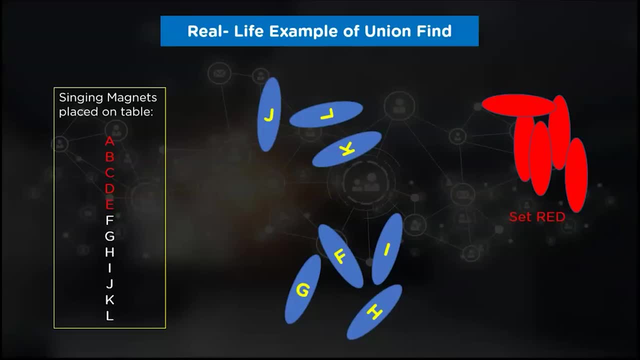 field, which will cause the bonding or connection of all these magnets. As a result, the magnetic field will be grouped together. We will now color code this set with red color. Along with that, we will also call this set as red. After that, the magnets F to I are also closer. 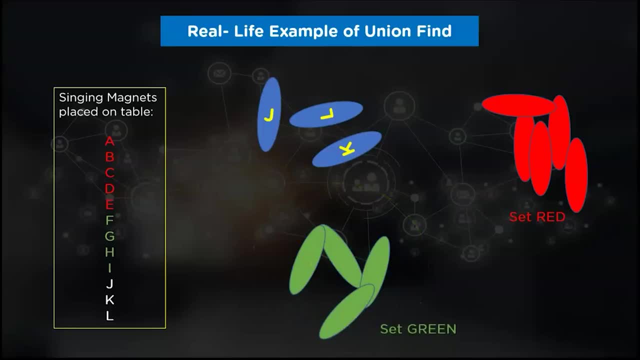 to each other. Thus they will also form a connection. We will call this set as green. Finally, this last set of magnets will also formulate a connection with each element inside a group. We will call this group, as said, purple E. All these distinct magnets got distributed into three different disjoint sets. 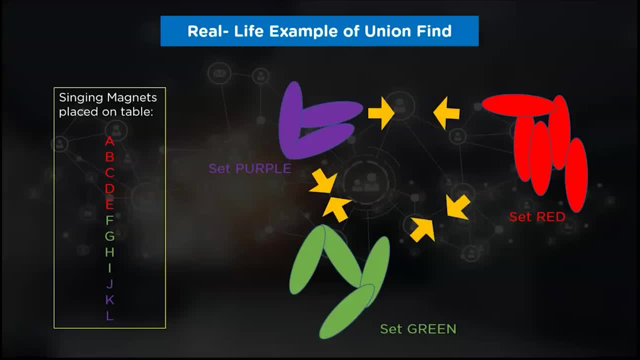 But as the magnetic attraction between these groups increases significantly, hence all these clusters of magnets will end up connecting with each other. This scenario can be related to the union function. Union function merges different sets into a single subset, where the find operation helps in extracting the group of element to which the particular element belongs. 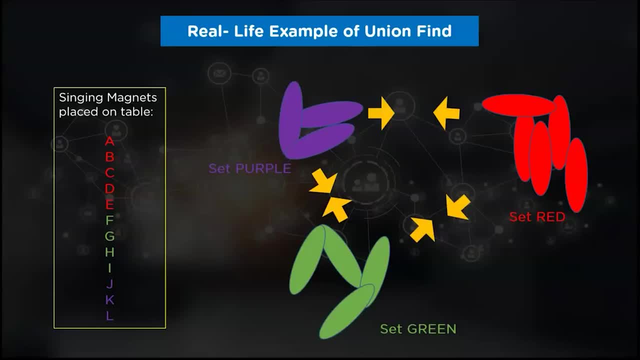 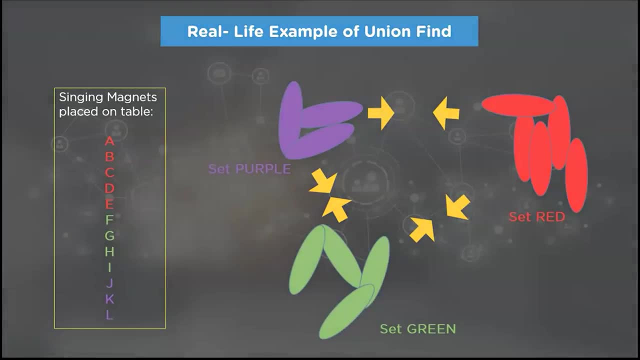 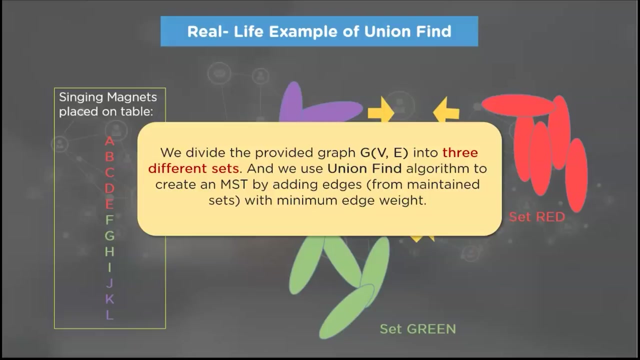 Similarly, in this scenario, a particular magnet can be traced back to its group with the help of color code that we have maintained alongside the magnets. The use of union find in Kruskal's algorithm can be related to this example. While implementing Kruskal's algorithm, we are going to maintain three distinct disjoint. 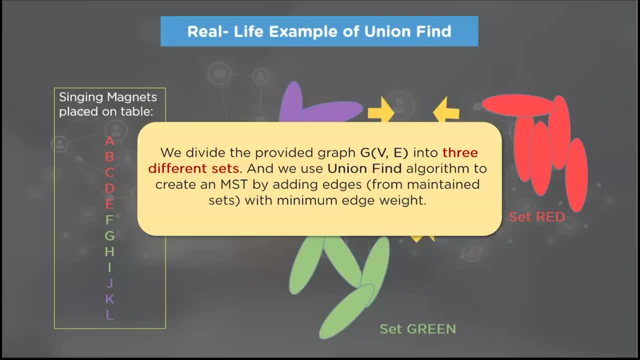 sets. The first set will store H-weight values for all ages in a graph, whereas the second set will store tree hierarchy for a different nodes. The last set will store H-weight values for all ages in a graph. The last set will store the ranks for all nodes included in an MST. 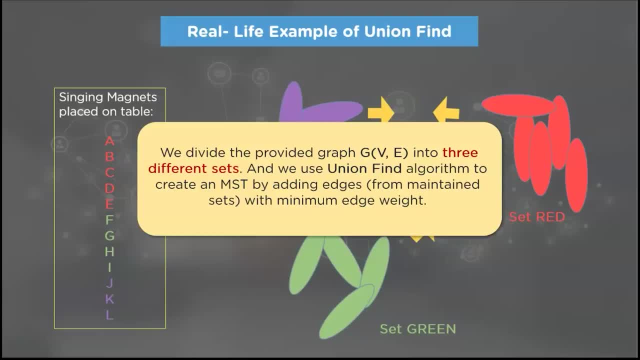 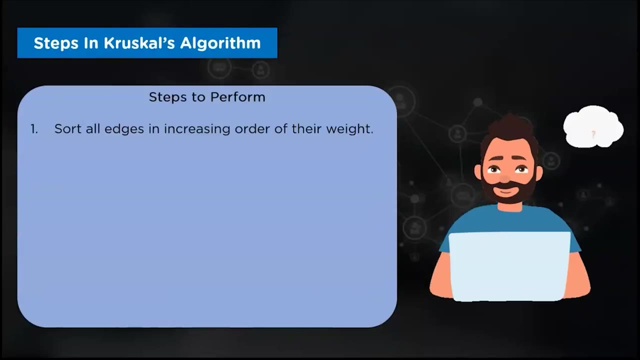 By using the union find structure and its operation. we can justify the entry of each age into the spanning tree, which we will explain in the implementation of this algorithm. But let's understand the functioning of this algorithm primarily. The Kruskal's algorithm begins with sorting all ages into increasing order of their age. 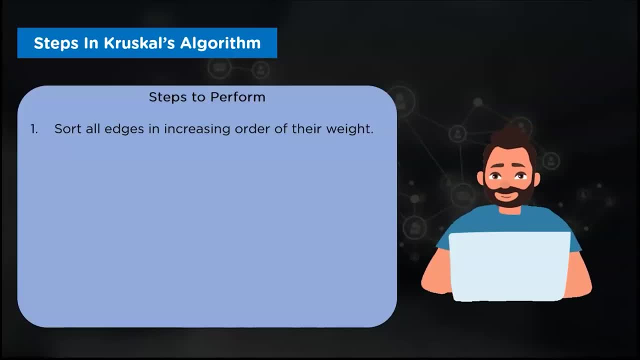 weights. This sorting is done to include ages with the least age weight primarily. This sorting is done to include ages with the least age weight primarily. This sorting is done to include ages with the least age weight primarily. After that, we'll pick the first smallest age and we'll check if it generate any cycle. 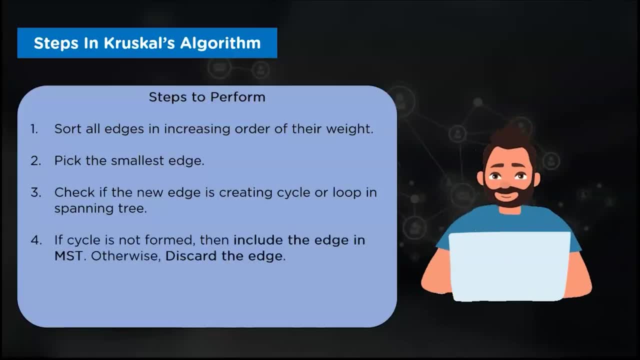 in the tree structure or not. If it does not form any cycle, then we will include that age into our spanning tree, otherwise we will discard it. We'll keep repeating this process until more than V-1 ages are included into our MST. 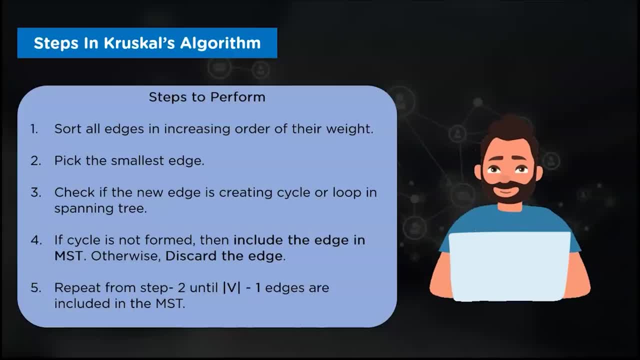 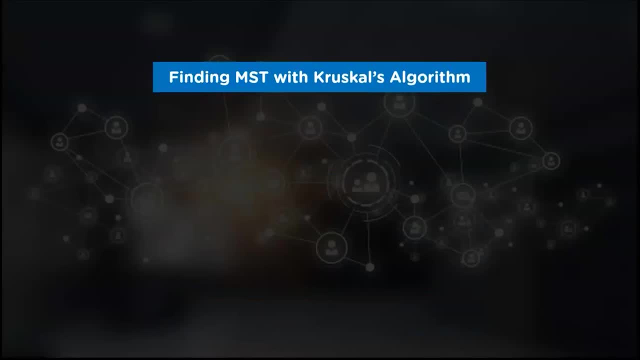 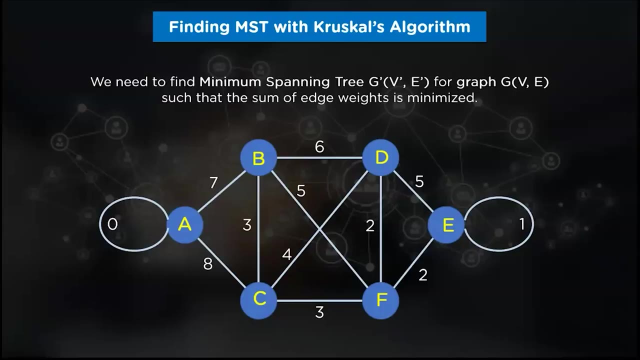 where V is the number of vertices. Now, moving ahead, Let's discuss how we can create a minimum span tree. So how can we create a minimum spanning tree with no age weight spanning tree? using Kruskal's algorithm, This given graph, GVE, contains 12 edges and 6 vertices, and we are supposed to find out. 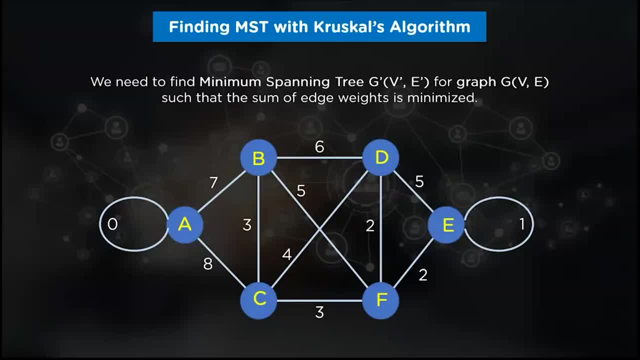 G', such that the number of vertices is equal to 6 and the number of edges is equal to V-1, that is, 6-1, which is equal to 5.. The one more condition that the formulated structure must abide by is that the summation 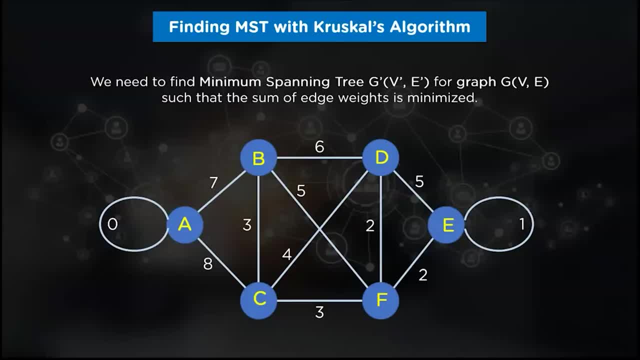 of all included edge weights must be the minimum possibility for this spanning tree. Going forward, we will discuss how we are going to create MST for this graph using Kruskal's algorithm. The first step that we need to perform is removing all the loops or parallel edges from. 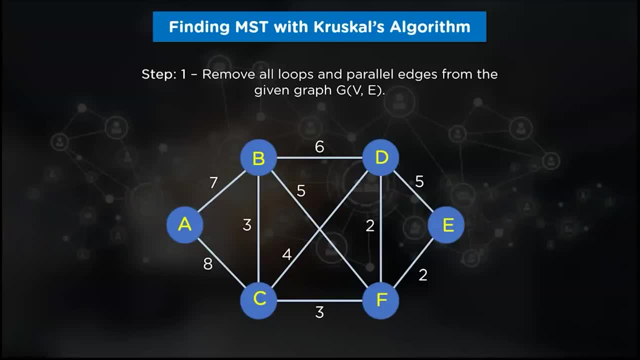 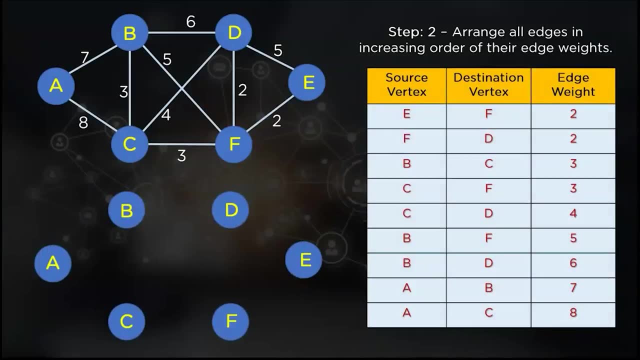 our graph. Hence, primarily, we will remove these two present loops. The next step that we are going to perform is arranging all the edges in increasing order of their weights. The reason behind maintaining the sorted list is to make sure that the first edge for 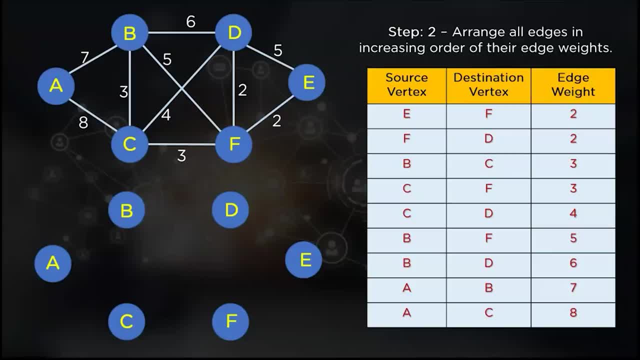 insertion is of a minimum cost. Here I have maintained the sorted list for all the edges that are part of our graph. So according to this sorted list, the first edge that we are going to insert in our MST is H-EF, as it has minimum weight cost, that is, 2.. 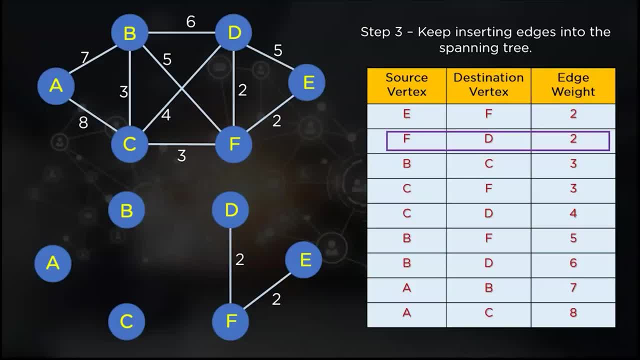 The next edge that we have in our sorted list is H-FD. It also has an edge weight equal to 1.. Hence, the first edge that we are going to insert in our MST is H-EF, as it has minimum weight cost, that is, 2.. 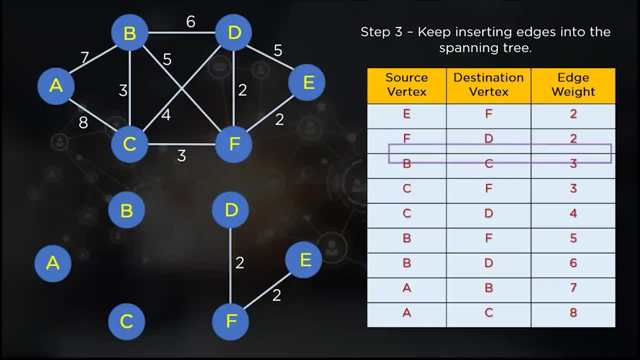 Hence we will include it in our spanning tree. The third edge in our sorted list is H-BC with weight 3.. The inclusion of this edge does not formulate any circle in our tree structure, hence we will add it to our MST. 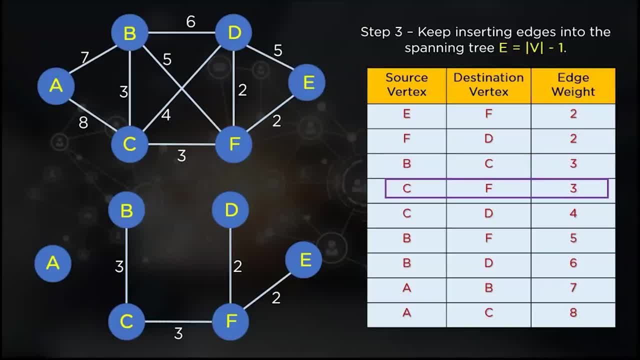 The next edge is H-CF having an edge, weight 3.. So we will include it in our MST structure. The fifth edge that we are going to pick is H-CD having weight 4.. But the inclusion of this edge inside our spanning tree will create a loop and the 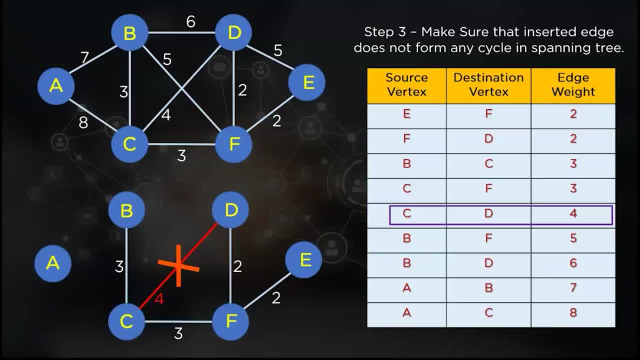 structure that contains a loop can never be considered as tree. Hence we have to exclude this edge. The next edge is H-BF, and the inclusion of this edge will also generate a cycle in our spanning tree structure, So we will exclude this edge as well. 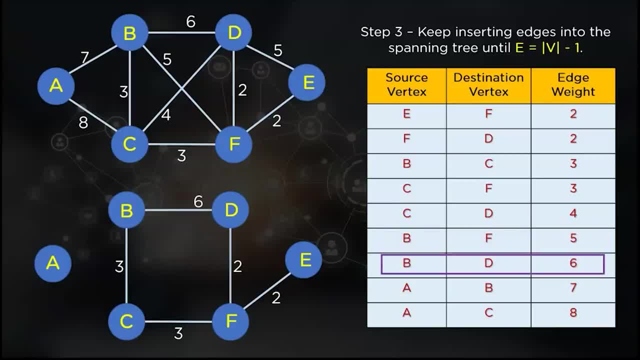 The next edge is H-BD. This edge has weight value 6.. The inclusion of this edge can also create a loop in our structure, So we will have to discard this edge as well. The next up is H-AB, with a weight value 7.. 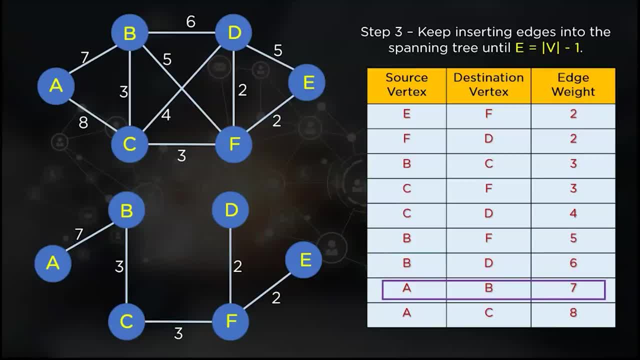 Even though this edge has higher weight value than previous edges, but it does not formulate any cycle in our MST, So we will include it in our tree structure. By doing that, we have generated V-1 edges, Hence we have to exclude this edge as well. 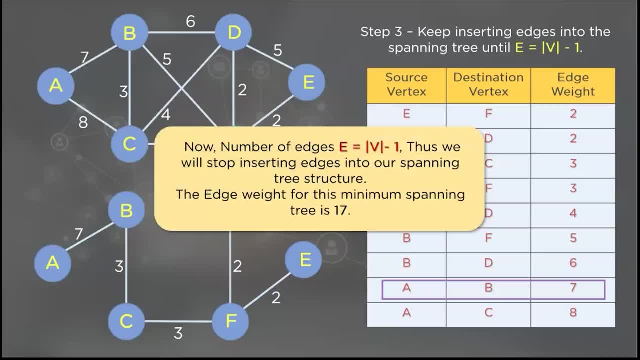 Thus we won't iterate further in our sorted list. This generated MST has minimum possible cost for our graph G-V-E, which is 17.. I hope that you guys have understood the MST implementation process using Kruskal's algorithm, Cause in the next slide I have a problem for all of you guys to assess your understanding. 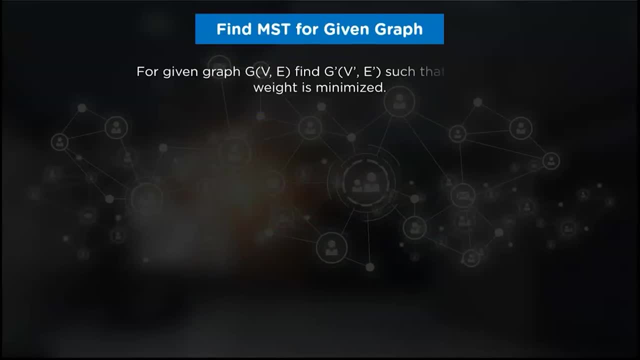 of Kruskal's algorithm. The graph shown on your screen contains 10 vertices and 18 edges, So we have to exclude this edge And for this graph you are supposed to generate a minimum spanning tree such that it contains 10 vertices, 9 edges and minimum construction cost. 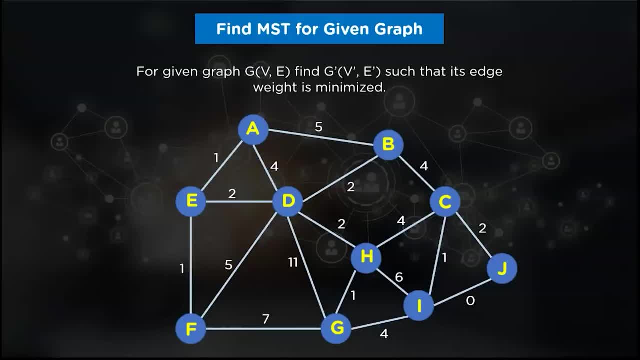 In order to do that, you can take out your pen and paper to draw the spanning tree structures based on the state that we have discussed till the time. I am aware that this graph is quite strangely structured. However, if you can solve this problem, you will undoubtedly be able to solve other difficult. 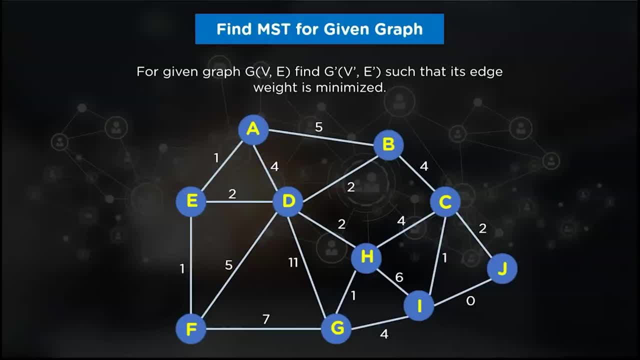 problems out there And, of course, if you are confused about any step, then you can re-iterate through the session. But here I am going to give you guys a little moment to figure out your answers. So let's get started. 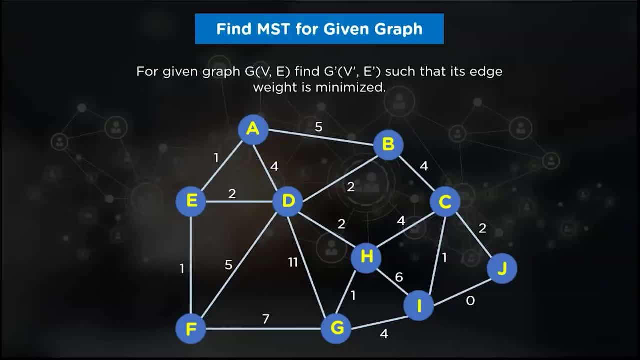 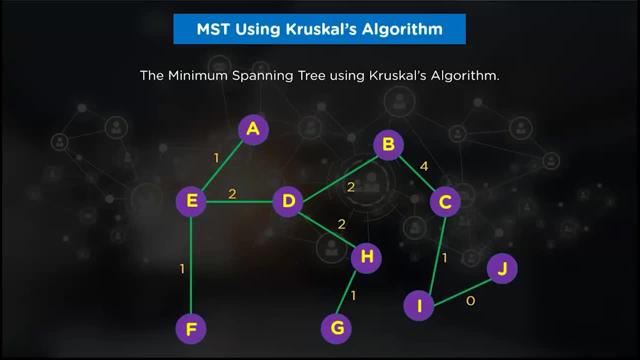 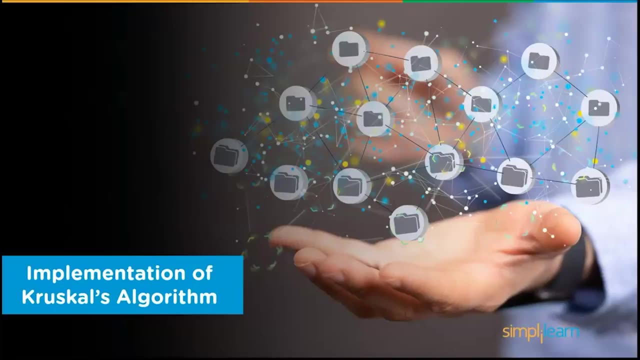 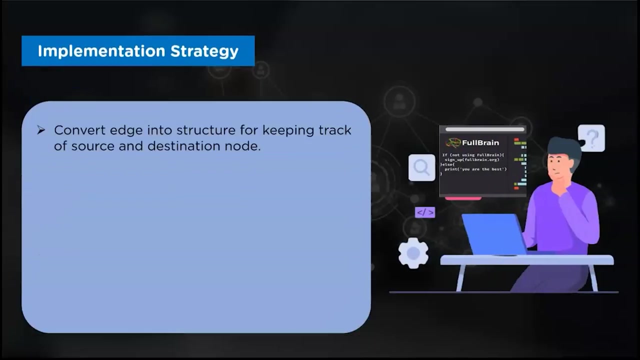 cost By removing other edges. the MST will look something like this: I hope you guys have got the right idea, So let's get started. Let's dive further and discuss the implementation strategy for Krouskal's algorithm. While implementing the Krouksal's algorithm primarily, we'll generate a C structure for 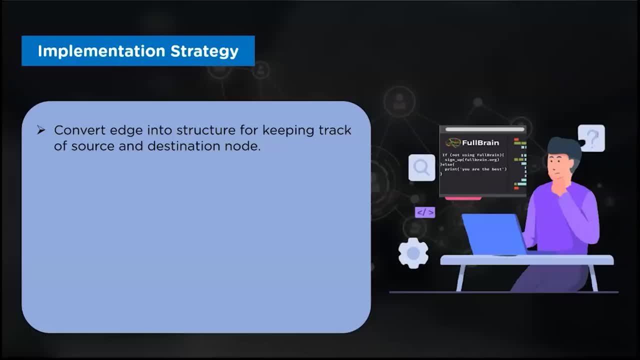 keeping track of the source and destination node, along with its weight. After that, we'll sort all the edges of a graph in increasing order of their age weights. Moving ahead, we'll create three distinct sets of the edges and the ∞, √, ÷, etc. 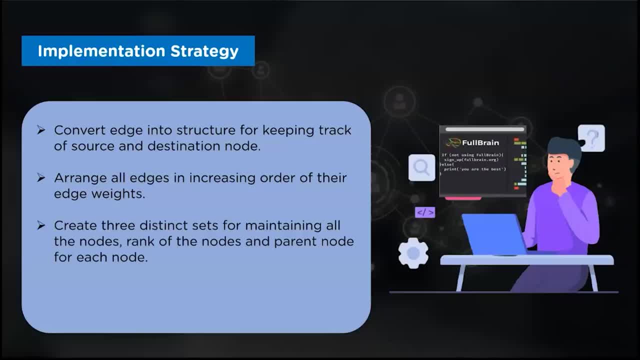 Here too, when you run paste, you will be able to get a formula that means the matrix is running out of time. distinct sets to maintain nodes of a graph, their hierarchy in tree and corresponding ranks for every node. For each insertion of an age in MST, we will 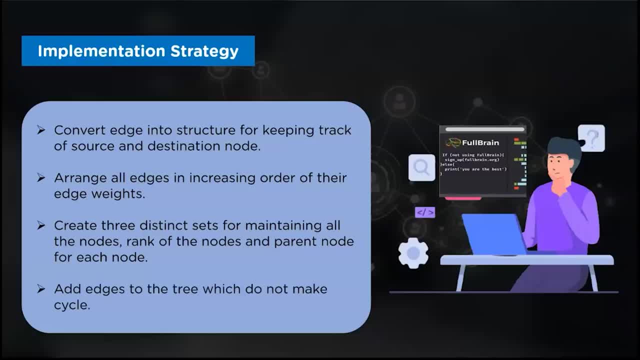 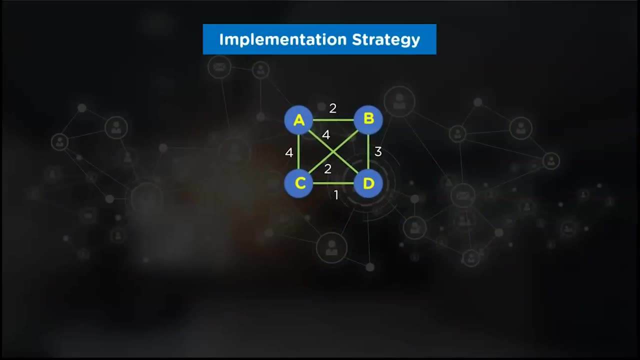 update the rank and parent of each node. If the two nodes have the same parent node, then we will not insert the age joining them, as it will generate the cycle in tree structure. Let's understand all these steps with the help of an example. This is the graph structure for which we will try to generate a minimum spanning tree using. 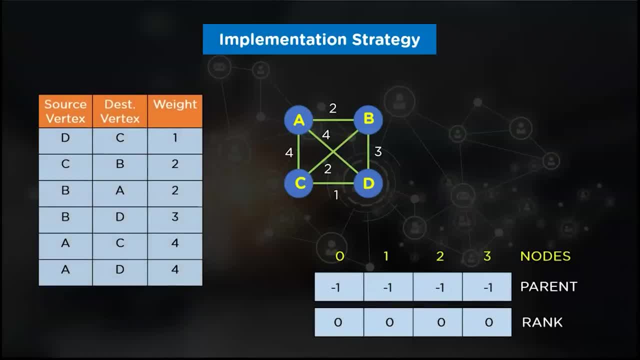 C programming language, As discussed earlier. primarily we will create a sorted list of all ages in increasing order of their age weights. The list will contain the source node, destination node and corresponding age weight for that particular age. Along with that we are going to maintain disjoint sets to carry out union operation. Those disjoint 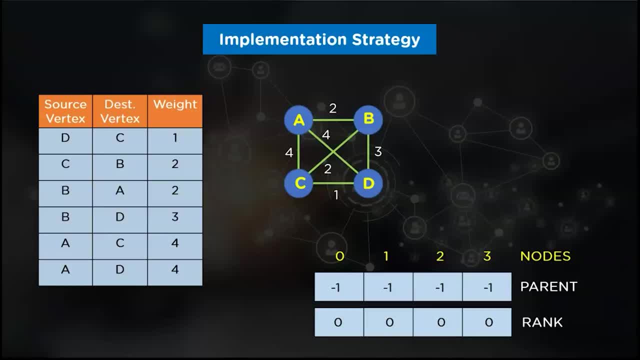 sets are parent and rank, And they will include the number of rows, the number of rows of the total data, the number of rows of the total data, the number of rows of the total data And also the number, rank value and parent value for every node in our graph. Initially, all the nodes are: 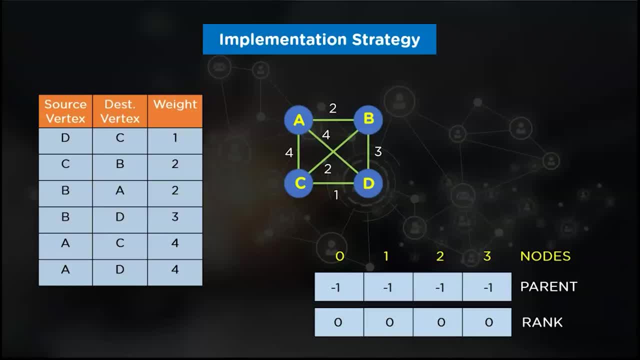 in their own different sets. Hence, we'll set their parent values to minus 1.. Also, the ranks for these nodes will be initialized to 0 at the beginning, because we haven't included them in our minimum spanning tree. Having said that, let's include the nodes. 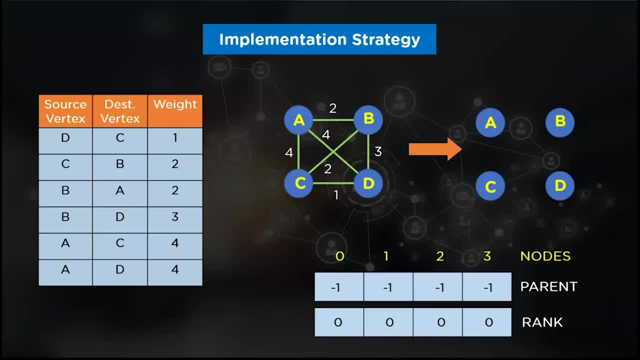 of our graph in our MST. In upcoming slides we'll traverse through our list of edges to include them in our minimum spanning tree. Now, the first edge that we are going to check is edge DC, which have minimum edge cost: ie 1.. In order to insert this edge in our MST, we'll need to find the absolute parent of 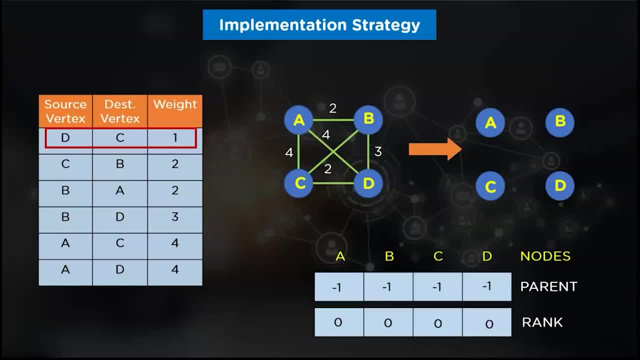 node D and C as well. So let's check out the parent set to determine the absolute parent value of node D and C. The parent value of node D is minus 1 and parent value of node C is also minus 1.. Both of them are having same ranks, Which means either we can make node D point to 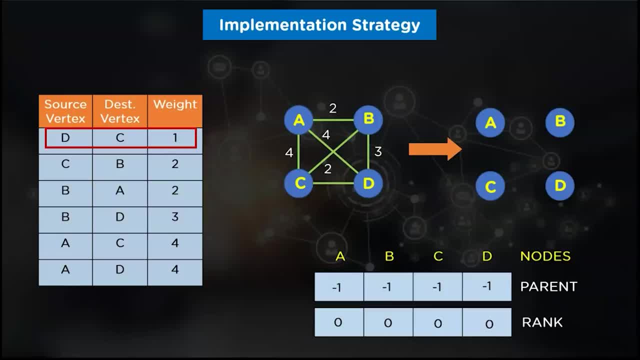 C or node C point to D. Here I'll assume that node D points to node C. So if node D is pointing to node C, then the parent of node D will become node C, And as C becomes the parent of node D, the rank of node C will change. 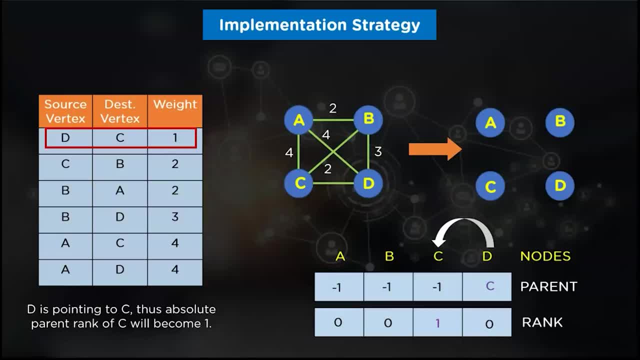 Remember, whenever two disjoint tree structures are joined together, then the rank of 1 being pointed to will increase by 1.. Hence the rank of node C will become 1. now, Once the disjoint sets are updated, the union operation will generate the link between node. 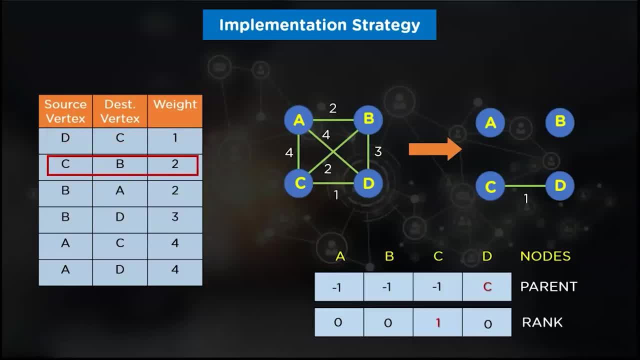 D and C. Now we'll process the second edge in our list, ie edge CB having weight 2.. Primarily, we'll check the parent values of both these nodes. Node B and node C have parent values minus 1 and minus 1. Which indicates that these 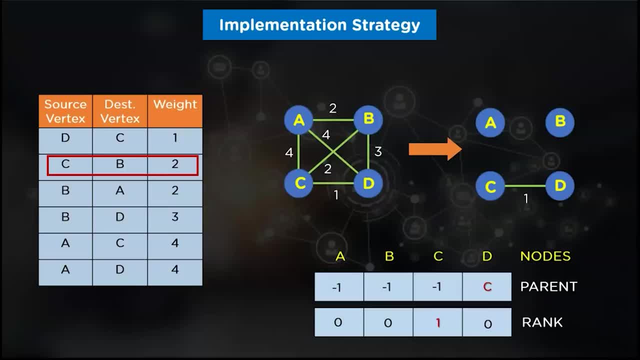 nodes are absolute parent of their own sets. Since they have different absolute parents, we can join both of them. However, the rank of node C is higher than node B. Thus the connection should point from node B to node C. As node B is pointing towards node C, the connection should point from node B to node. 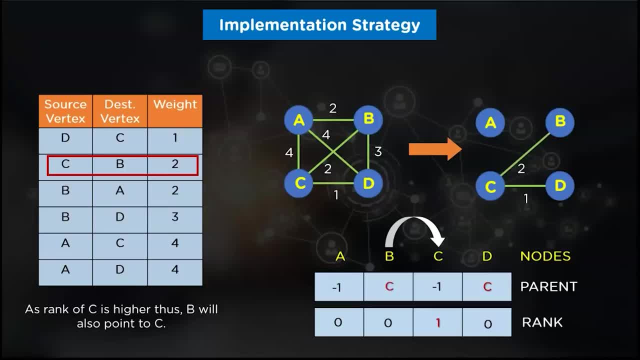 C. Thus node C will become the parent of node B as well. Hence we'll update the corresponding absolute parent values for them. Next up is edge BA with the weight value 2.. Now the parent value for node A is minus. 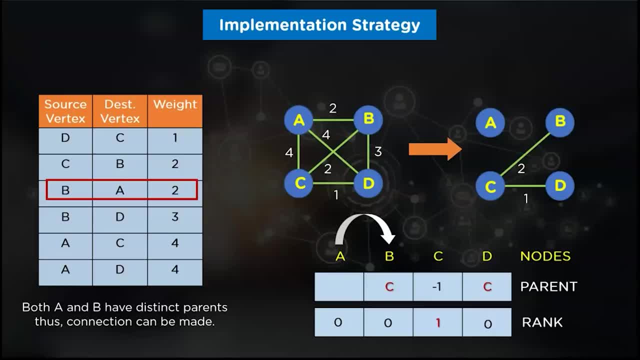 1 and the parent value for node B is C, So both of them have distinct parent value, Which implies that we can establish a connection between them. For that purpose, we'll have to update the rank of node B and node C, So both of them have distinct parent values. 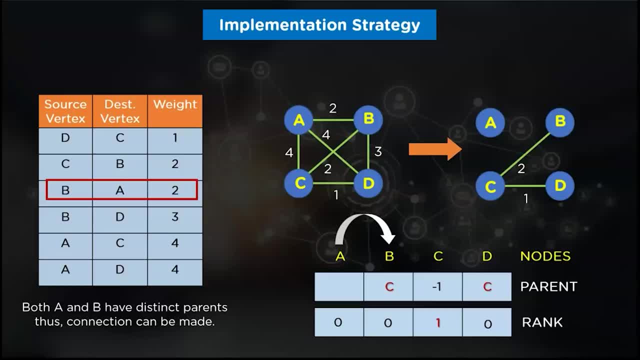 In the next step, we'll change the number of children in order to reduce the rank of the children. After that, we'll want to remember that we don't have to report one every lesson. In the next step, we'll ask our child to be a parent of one of the children. 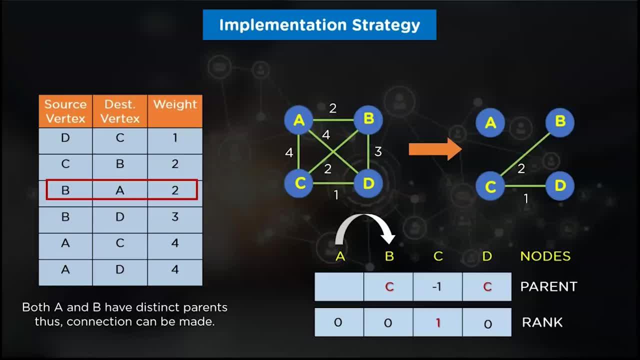 To do this, we'll update the rank field And, as the parent of node B is node C, the rank of C will definitely increase by 1.. Once the fields are updated, the edge will get included in our MSD. On that note, We have generated our minimum spanning tree. But you must be thinking about 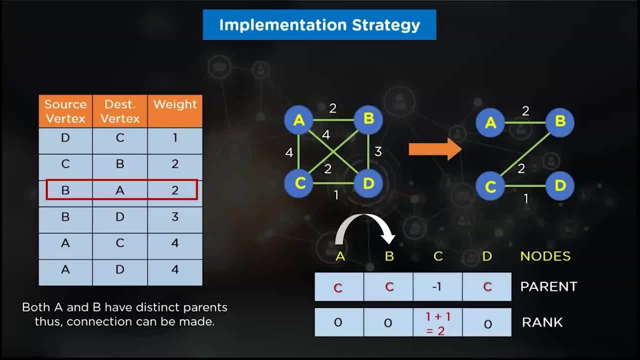 how our algorithm will discard the other edges. So to understand that we'll traverse further in our list of edges. The next edge is age B, Then the next age is age Z, AC, and the parent of node A is node C itself. Hence we'll discard this node as. 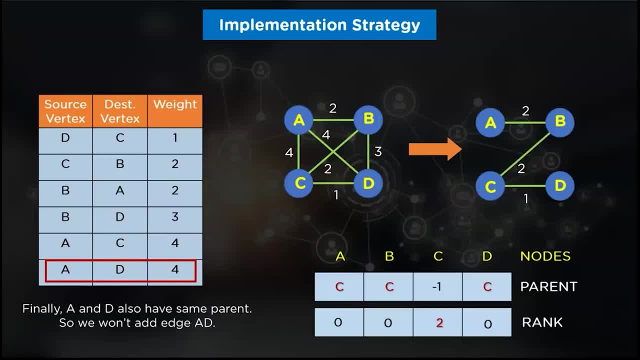 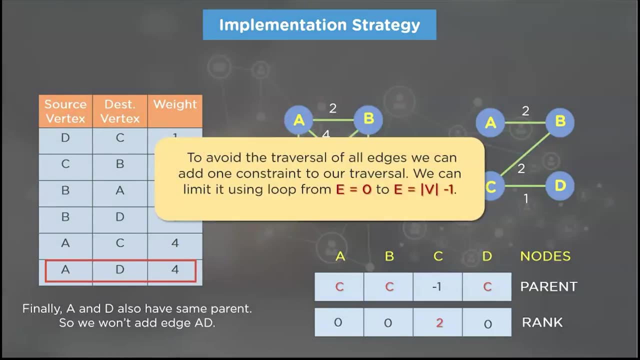 well, Now the final age in our list is age 80, and again both these nodes have the same parent node. Thus we'll discard this node as well. Now you must be thinking about how we can limit iteration of the whole list if we formulate MST using the few topmost ages only. Well, the answer to that is: 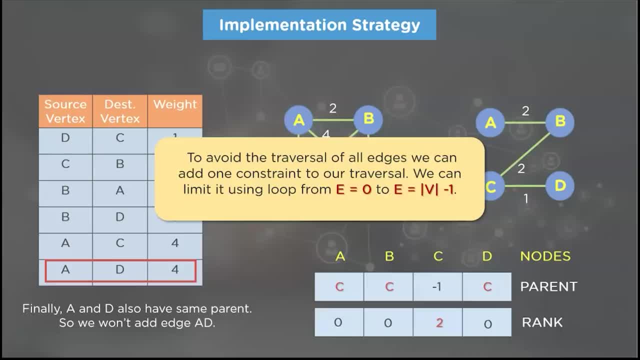 pretty straightforward. We can avoid the complete traversal of the list by using looping condition from E is equal to 0 to E is equal to mod of V minus 1.. When we use this condition, the looping will stop when V minus ages get included in our MST. Now the next ERP is the time complexity analysis of 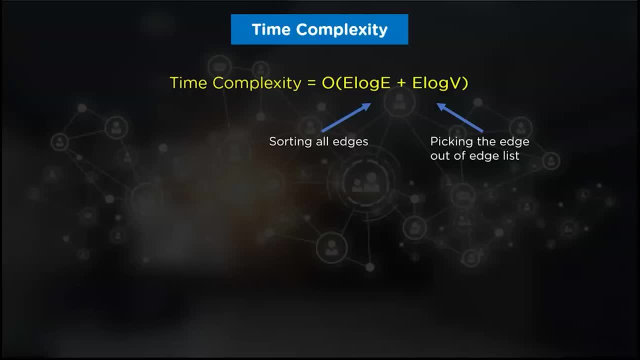 kurskal's algorithm. The time complexity analysis of kurskal's algorithm can beевич Piggyback's algorithm. complexity of Kruskal's algorithm will be big O of e log e plus e log v, The e log e for sorting all ages and e log v for finding the age from maintained three sets. The average time complexity. 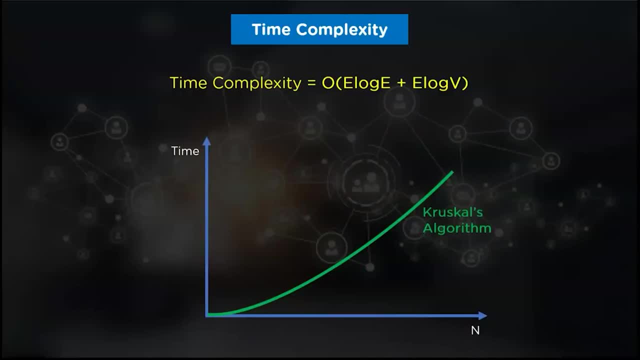 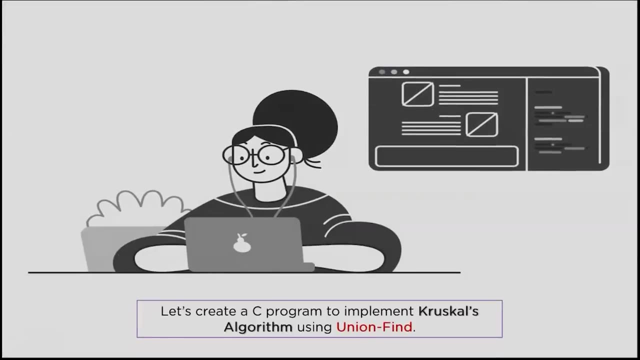 graph for this implementation will be something like this: It will be of parabolic nature. I hope that you all have understood the strategy for implementing Kruskal's algorithm. So, without wasting any time further, let's visit the code editor to develop a program in C programming. 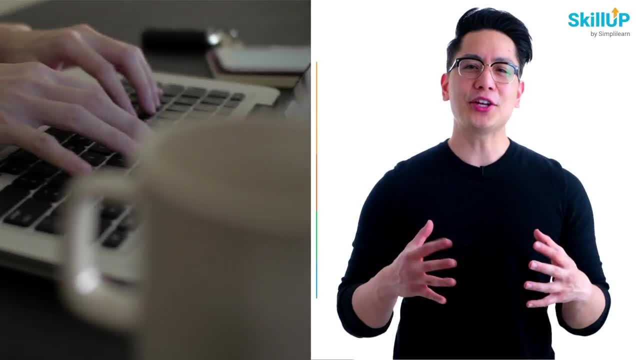 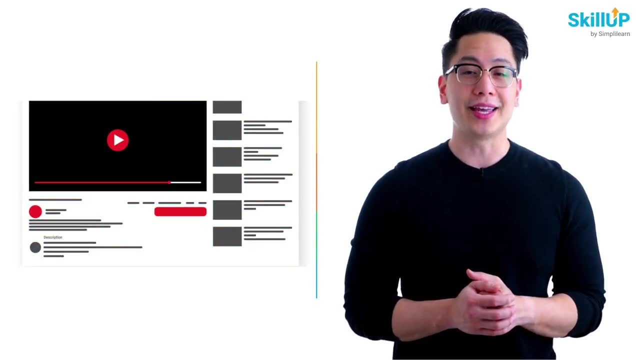 language for Kruskal's algorithm. If getting your learning started is half the battle, what if you could do that for free? Visit SkillUp by SimplyLearn. Click on the link in the description to know more. Now to begin with coding implementation, the first thing. 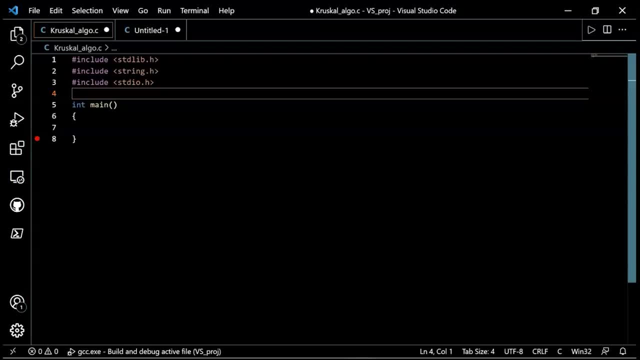 that we'll do is we'll create a storing system to represent a weighted age. For that purpose we'll use Storing Structure in the C programming language. So let's get started with that Struct age. and and said, this structure will create int source. 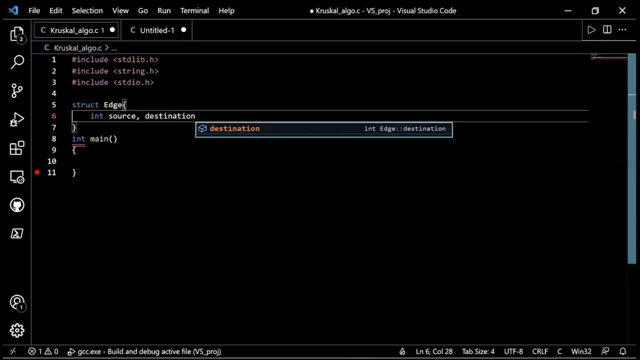 destination and wait. Now. what we'll do is we'll utilize this structure to store the ages of the graph. Moving ahead, we'll also initialize the structure for storing the complete graph. So let's create one more structure And we'll name the structure as graph. 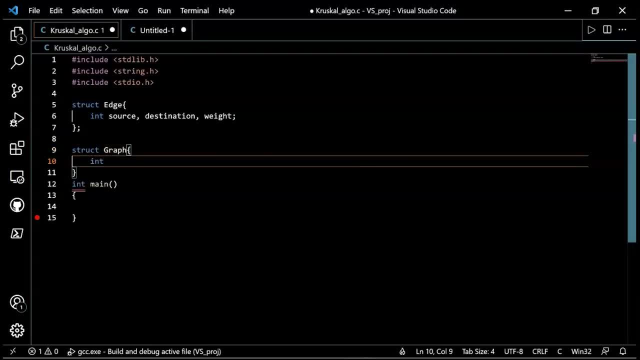 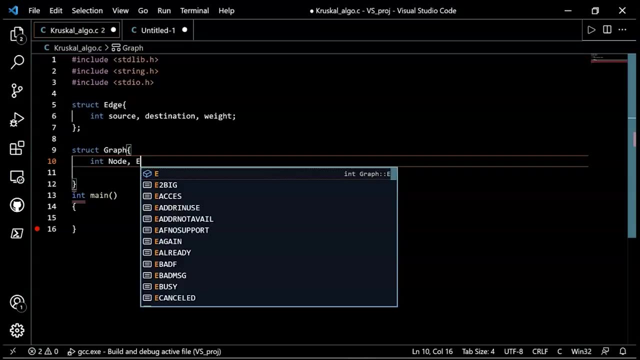 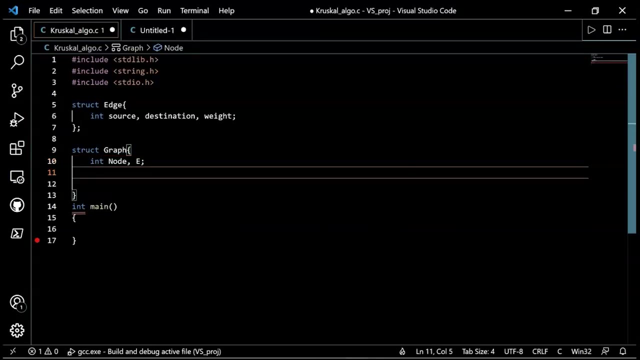 And inside this graph structure we'll create node. We'll also create variable E to represent number of ages in our graph. We'll also call the reference of structure age to this graph. By doing this, we'll be able to include all the ages into our graph structure as well. So let's create that reference struct age, star age. 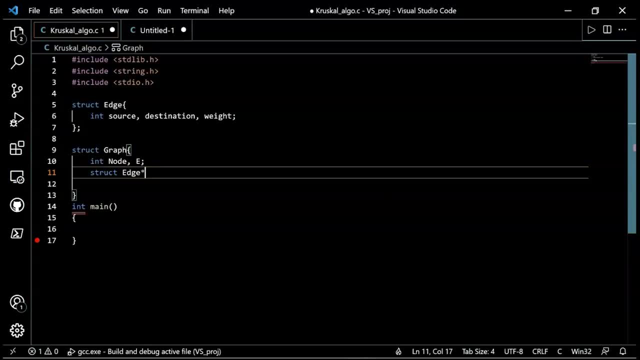 now, we have successfully created the structure for graph. now, moving forward, what we'll do is we'll assign dynamic memory to the reference of graph structure. for that, what we'll do is we'll write code, struct, graph. 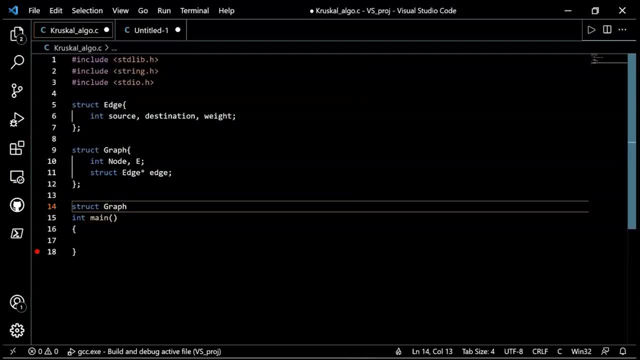 star, generate graph. and inside this function we'll pass int node and the number of edges, that is e variable. now we'll write body for this function and we'll write body for this function. and we'll write body for this function and inside body, first thing what we'll do is we'll create the space. 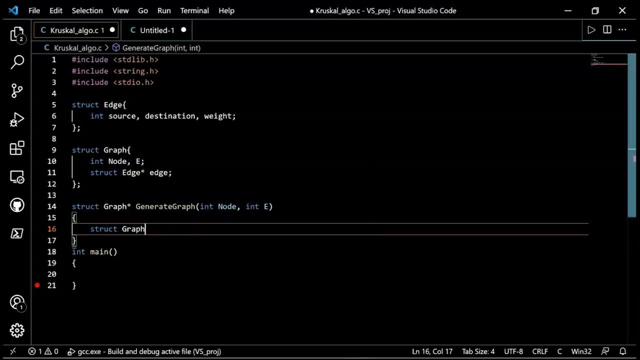 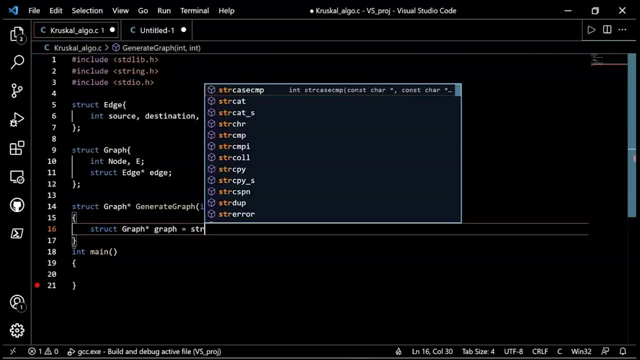 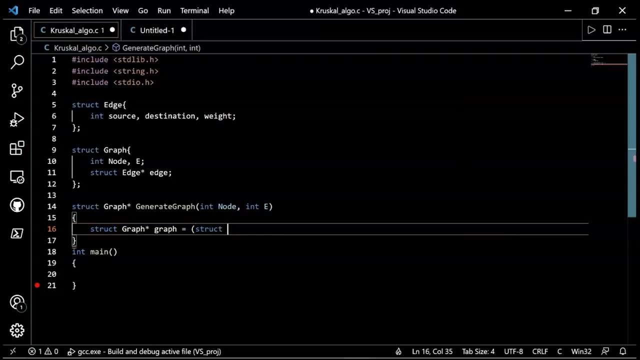 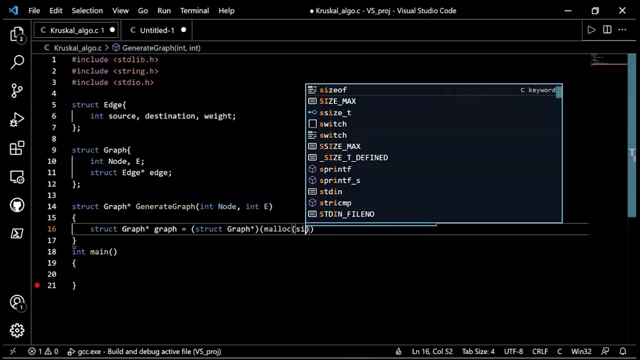 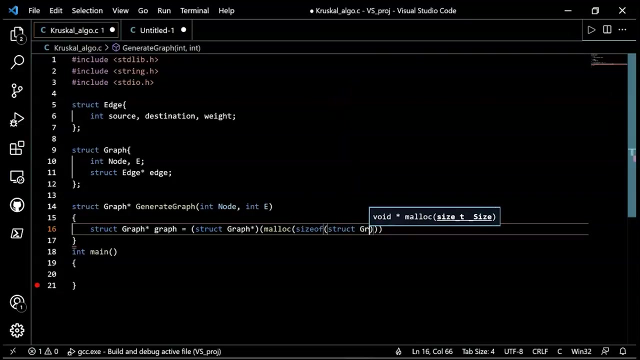 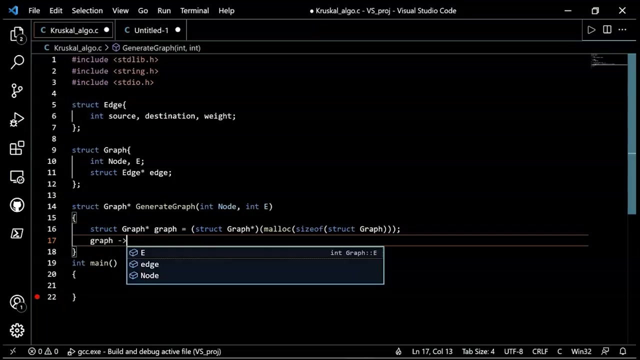 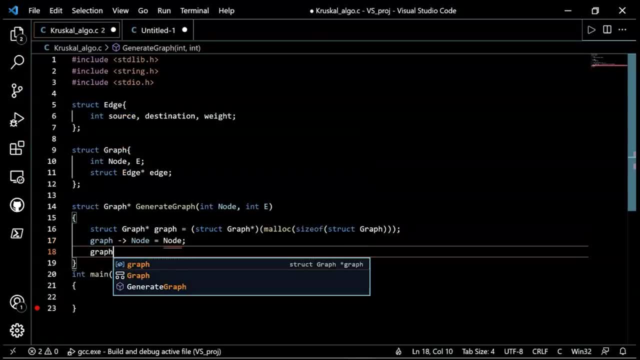 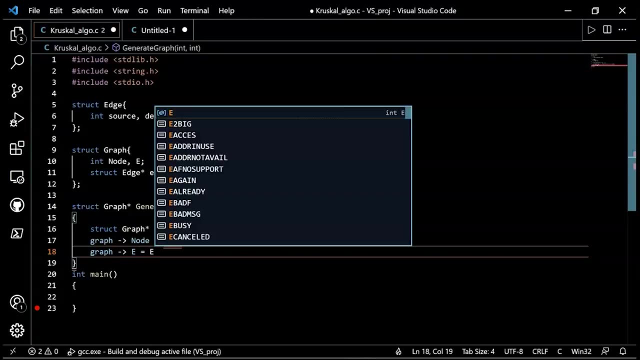 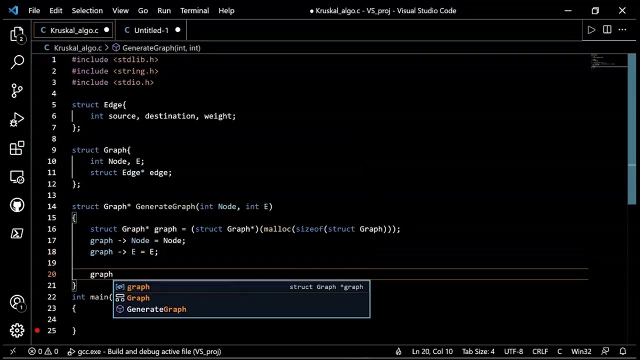 and graph nxt: dot. number of edges: dot. number of edges: dot. number of edges will be equal to e itself, to e itself, to e itself. next, what we'll do is: allows: we'll allocate a memory to each edge. okay, underscore here for that. what we'll do is: 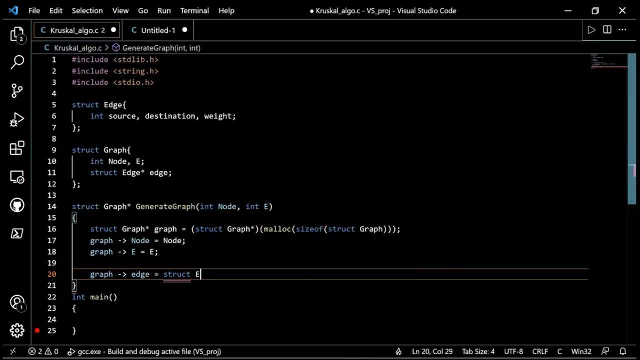 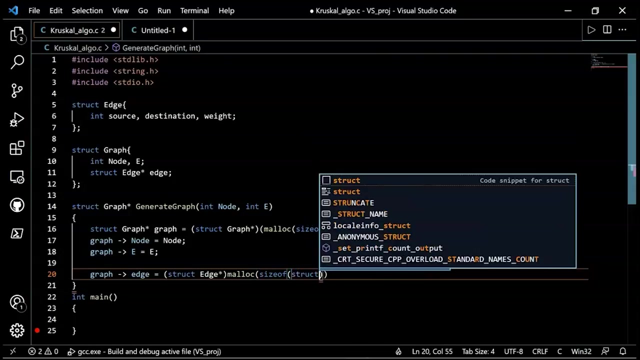 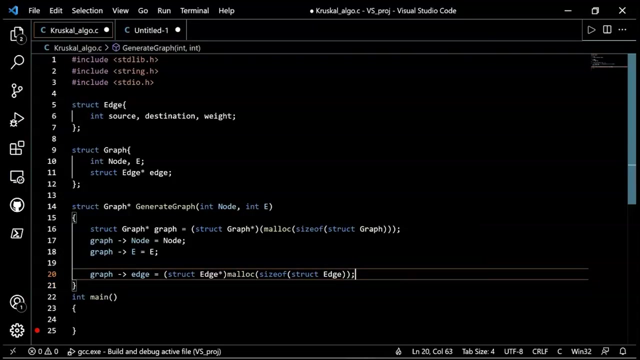 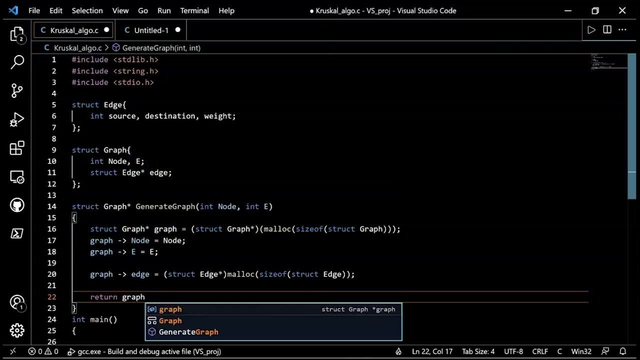 we'll use struct, edge, star, malloc, size of strut, age, age and, finally, we'll return the graph. now we have successfully allocated memory space to our graph and individual edges as well. so, moving forward, what we'll do is we'll initialize one more structure to store the parent array and rank array. basically, these are the. 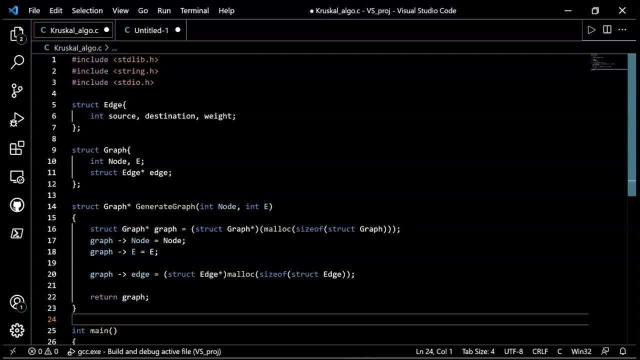 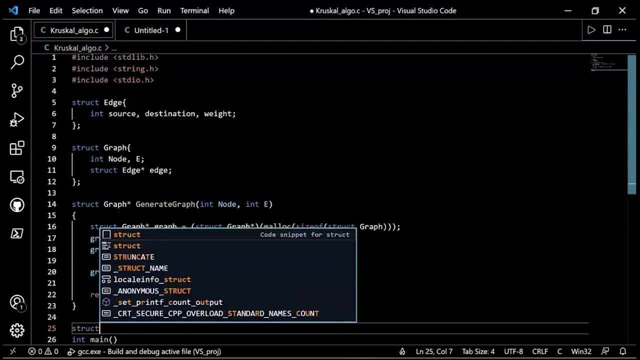 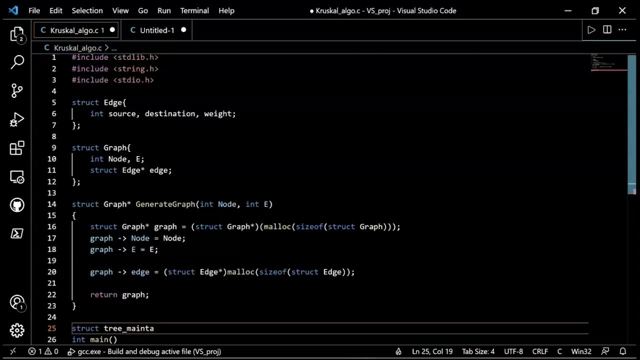 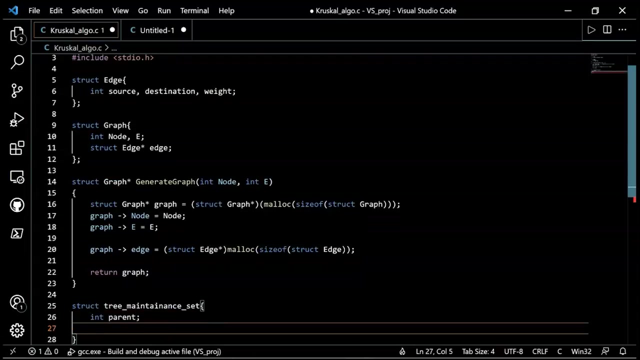 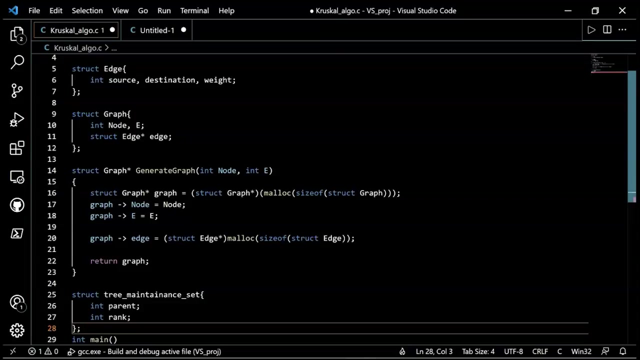 disjoint sets, whose usage will allow us to generate a spanning tree using union find algorithm. so let's get started with that. we'll create another structure and we'll name this structure as tree underscore, maintenance underscore set, and and said: this structure will create parent array and and rank array. now we have created the tree maintenance set structure, so let's. 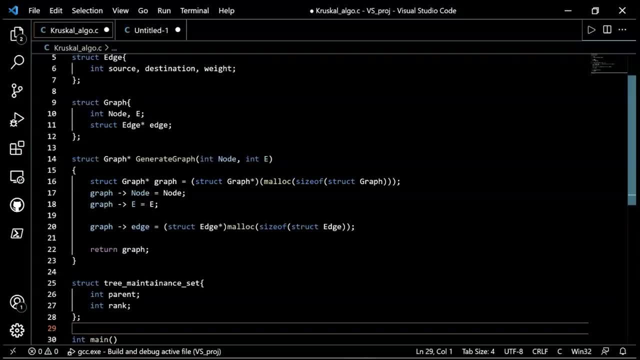 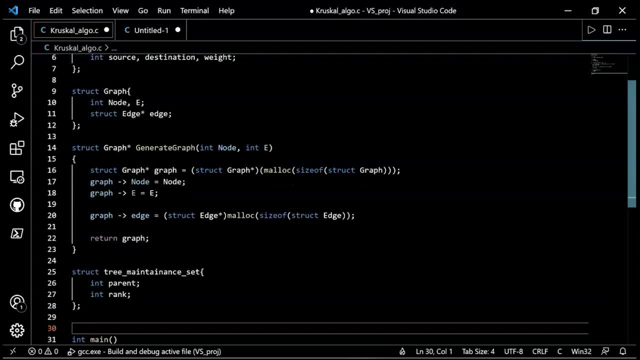 generate an union find algorithm for maintaining MST structure. in order to do that, let's create a function named find disjoint set first. so this find disjoint set function will be of int data type- find underscore- disjoint set, and inside this will pass struct tree underscore- maintenance underscore set. 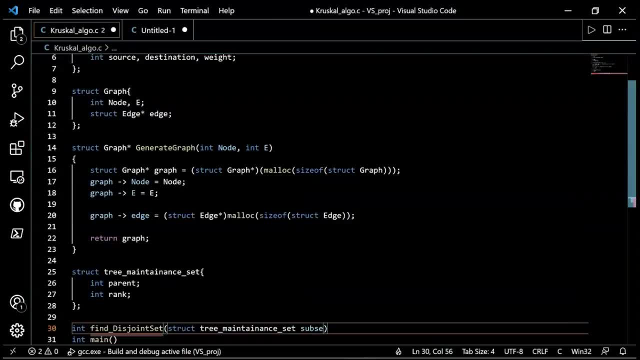 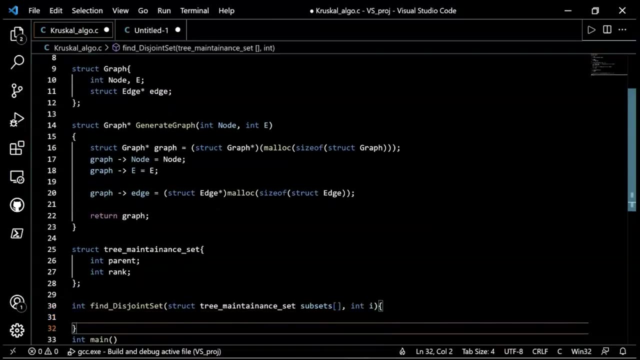 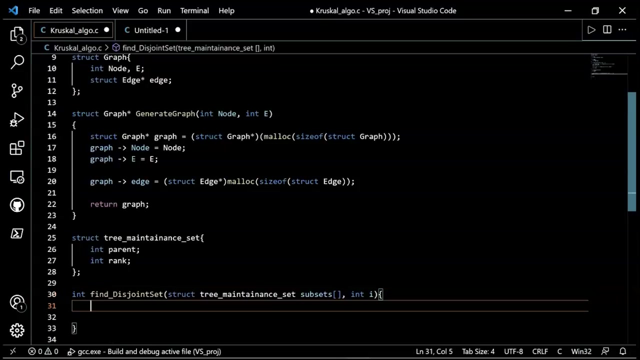 and it's object subsets and a variable int I inside this function will use its case to find root and make it as a parent of argument I. also, if it is minus 1, then we'll need to update it for that we'll keep recurring through this a block by calling the function find disjoint set inside a block. so 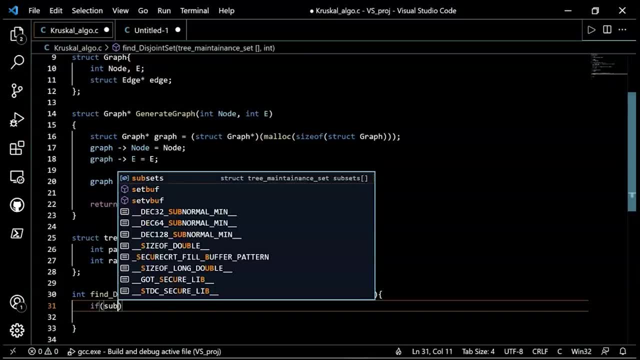 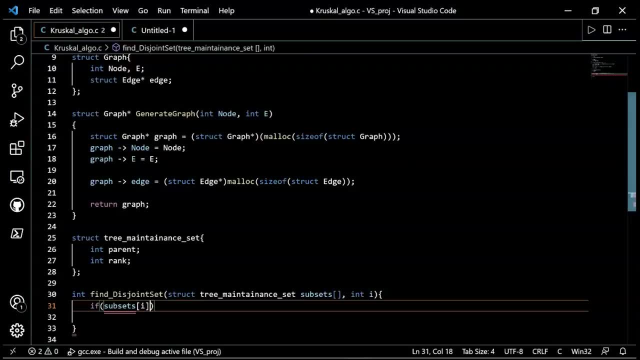 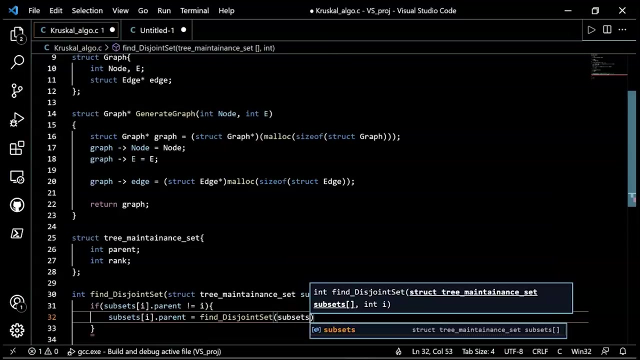 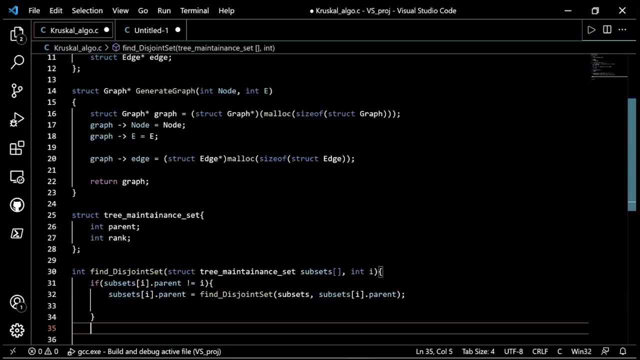 let's do that. if subsets I dot parent, it's not equal to find, to find underscore, disjoint set and will again pass same argument: subsets, comma, subsets i dot parent. and finally, we'll get out of this if block and will return subsets i dot parent, dot parent. 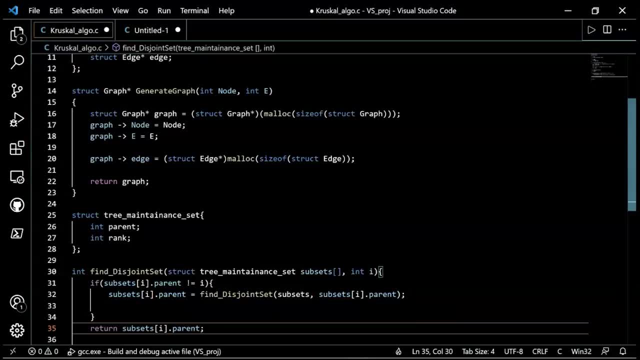 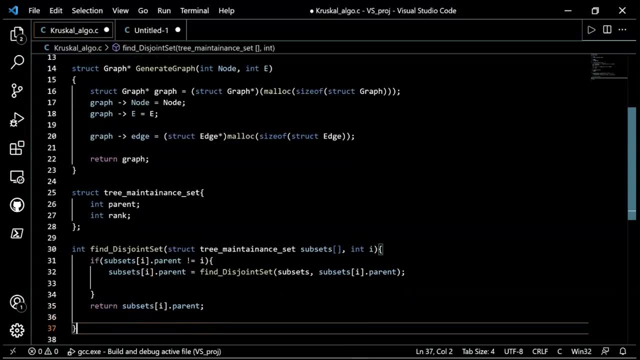 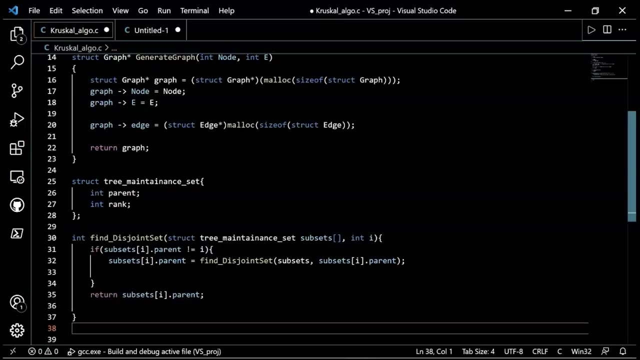 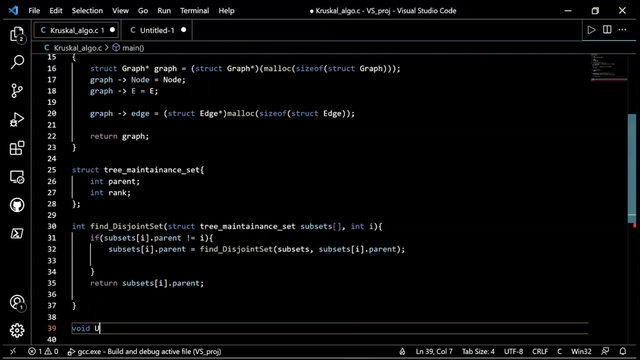 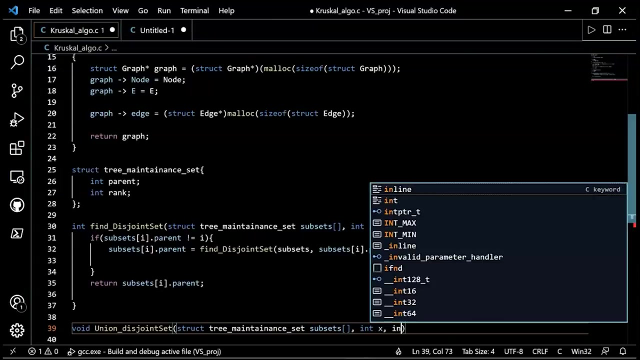 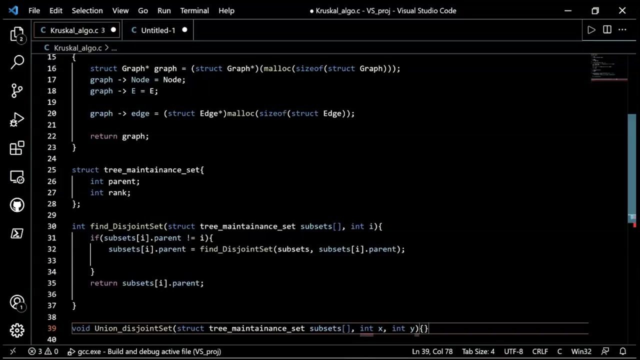 now we'll create a function for union operation. let's name this function as void union under union. underscore disjoint set and inside this will pass: struct tree underscore- maintenance. underscore set and its object subsets and its object subsets and its object subsets subsets set. row of argument x. 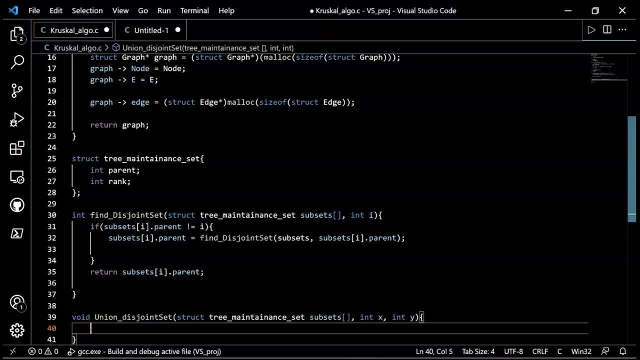 and argument y subsets and will pass argument x and argument y and the rear column, Palestine from from find disjoint set when the x has been passed to the function and similarly the y root will store the return value for find disjoint set, given y as an argument. so let's 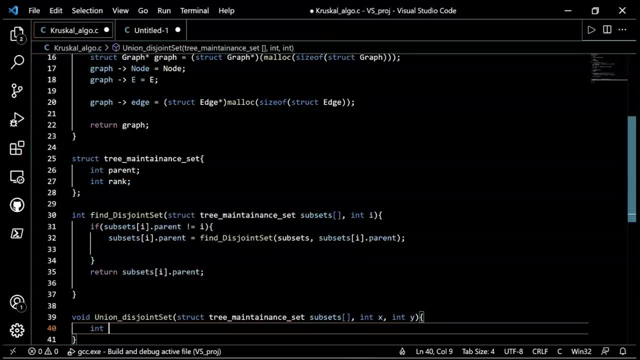 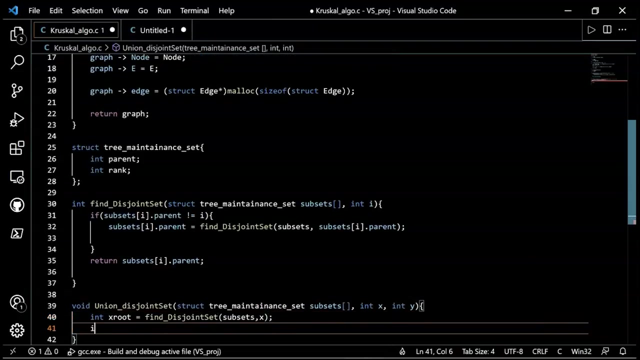 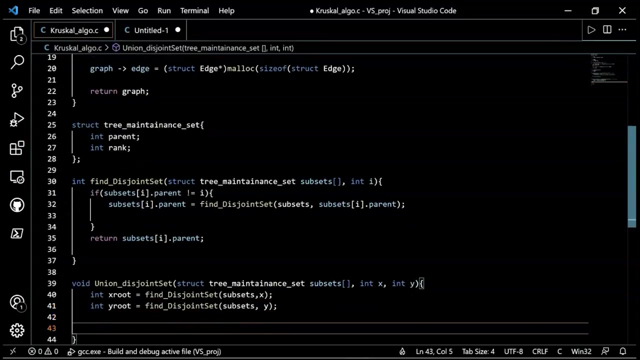 write command for that. end xroot will be equal to find disjoint set and objects will be subsets. comma x: Similarly, end yroot will be equal to find. Now. in order to build connection between these nodes, as discussed previously, the node with lowest rank value should always be pointing to the node with highest rank. 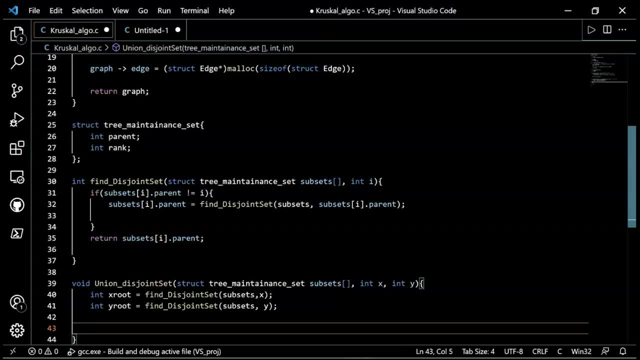 value and vice versa. So we'll have to use this if block in order to put this condition in the connection building block of our program. So we'll write condition for that here now. if subsets x, root dot rank, it's greater, less than subsets. 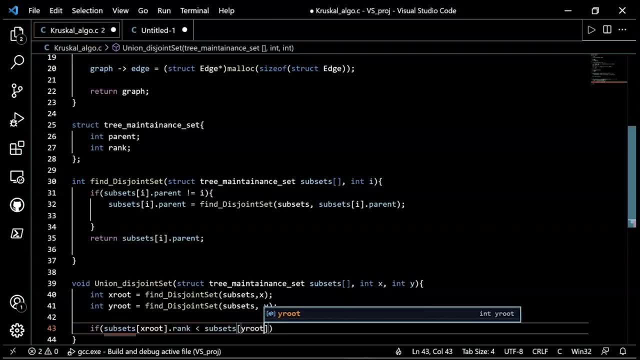 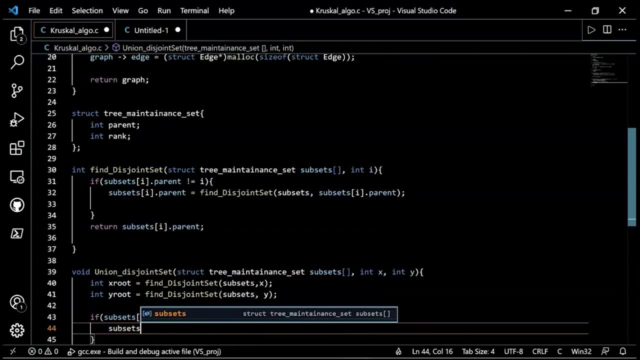 subsets y root dot rank, then what we'll do is we'll set subsets x root dot parent to y root. That means subsets. So what we are doing here is we are checking the rank value of x root If the rank value of x root is smaller than y root. 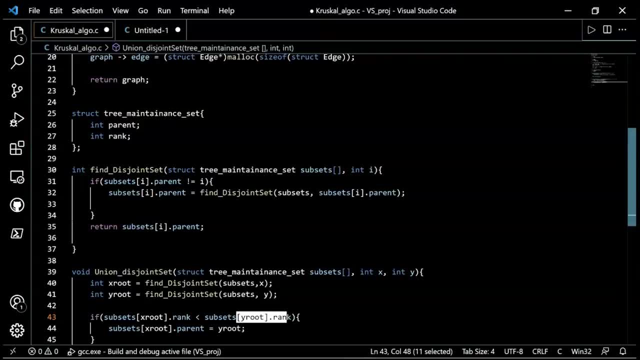 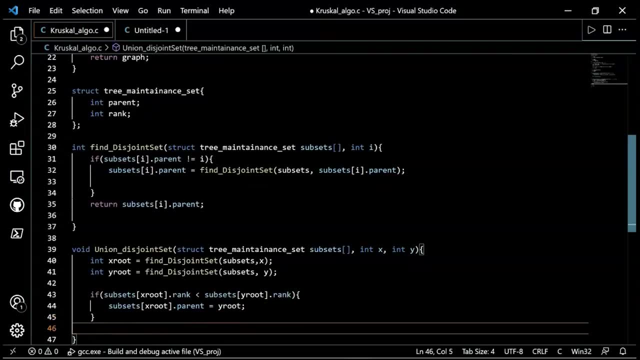 Then what we'll do is we'll simply set the y root as parent of x root. I hope you guys are clear with this. Now moving forward, we'll write else if part of this condition, else if subset x root dot rank. Sorry, I'll have to. 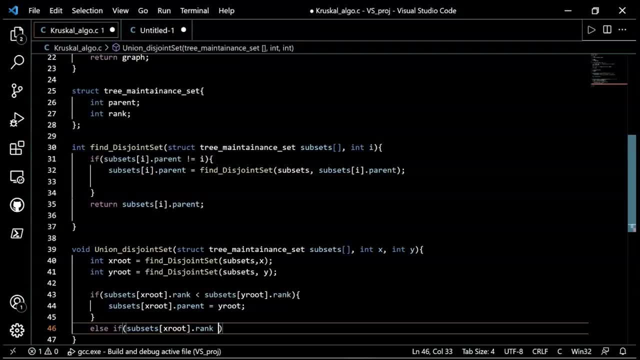 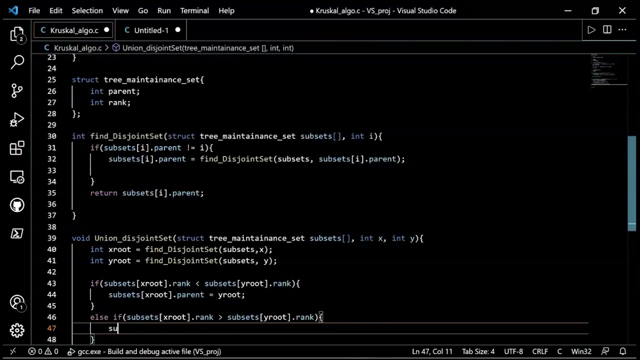 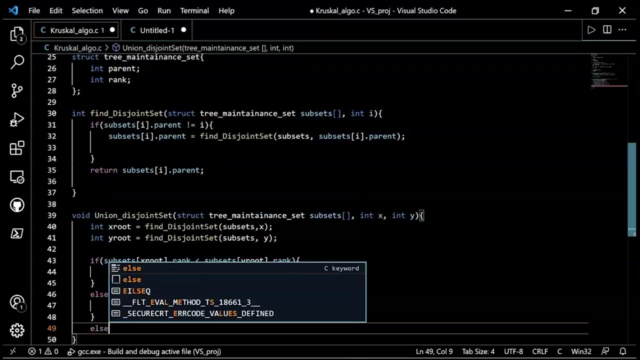 Let's see here: and if subsets x root dot rank is greater than subsets y root dot rank, then what we'll do is We will set subsets y root dot parent is equal to x root. otherwise, if both above mentioned condition fail, then what we'll do is we'll add one more condition: will set subset y root dot. 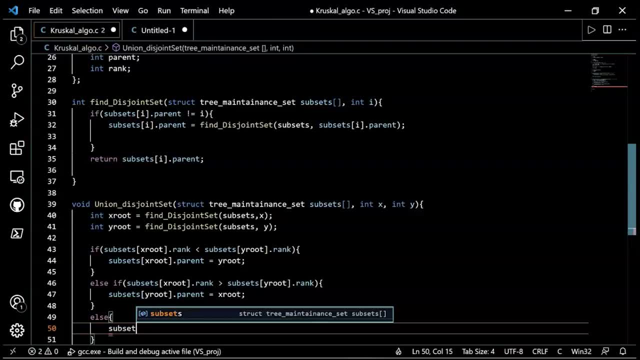 parent is equal to x, root. Otherwise, if both above mentioned condition fail, then what we'll do is we'll add one more condition, say: subsets x, y, root, dot. parent type post, click s düşün, Then we Set subset. 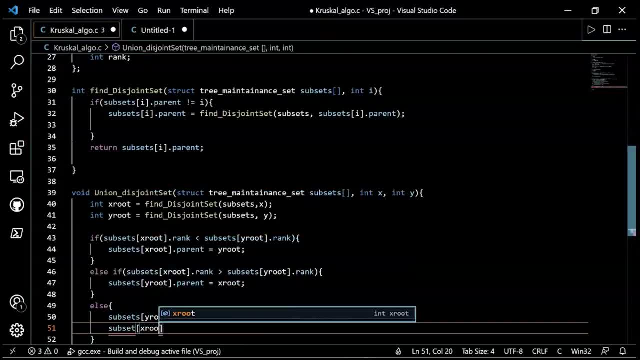 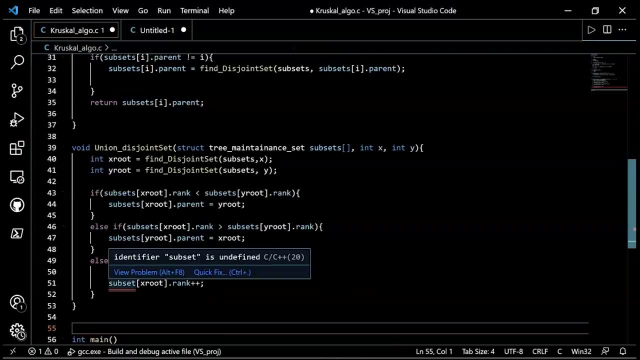 Sent subsets by argument X, root, root dot rank to incrementation. there is one mistake over here: subsets. okay, so now we have implemented the union find algorithm for the schools implementation. next we'll create a function to sort the list of ages in our graph according to increasing order of their age weights. 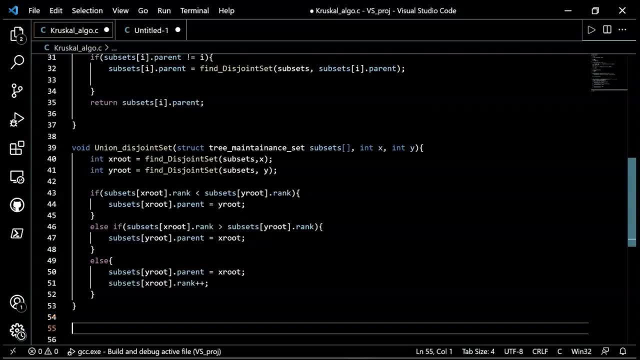 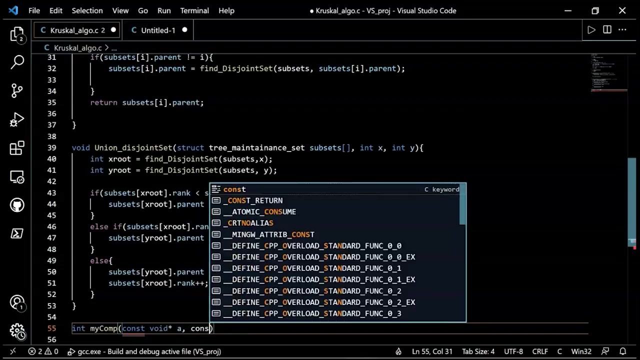 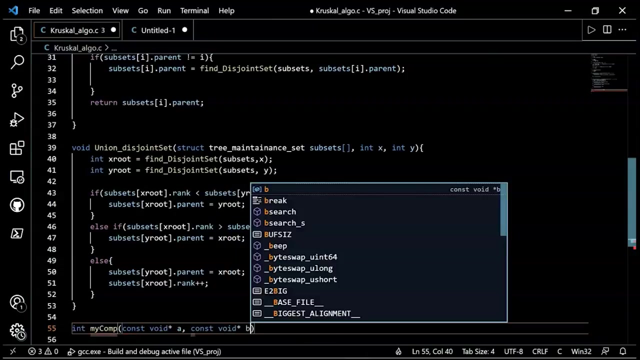 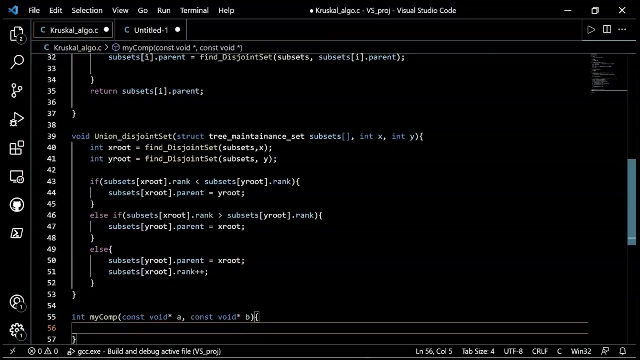 so let's create new function for that. we'll name this function ads and my comparator, and inside it will pass const void star a and const void star p and we'll create function body. but before we get started with coding implementation of this, my comparator function, i want to talk about arguments of this. 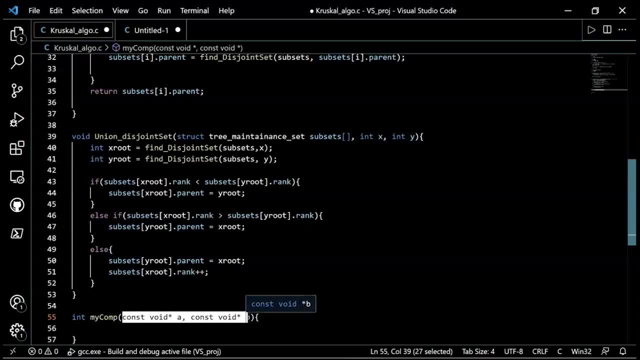 function. so, basically, a and b are constant quantifiers. the significance of this quantifier is to tell the user that you cannot modify this pointer and the location it is pointing to throughout the program. so let's get started with the coding part of this, my comparator function. what we'll do is: 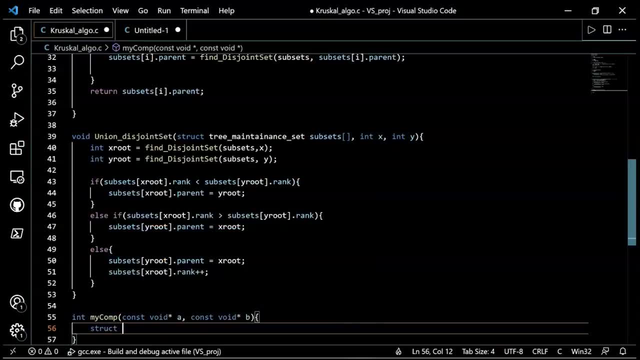 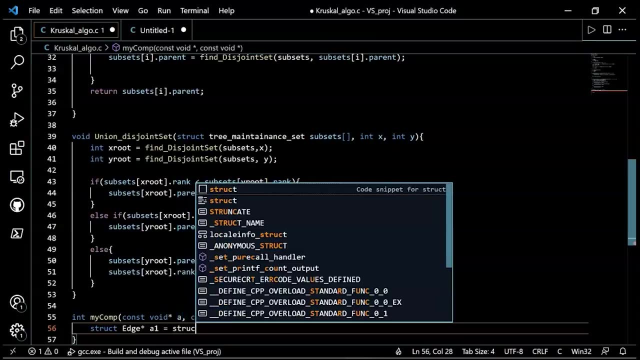 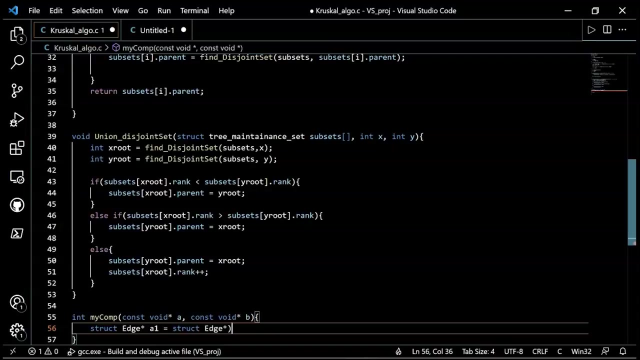 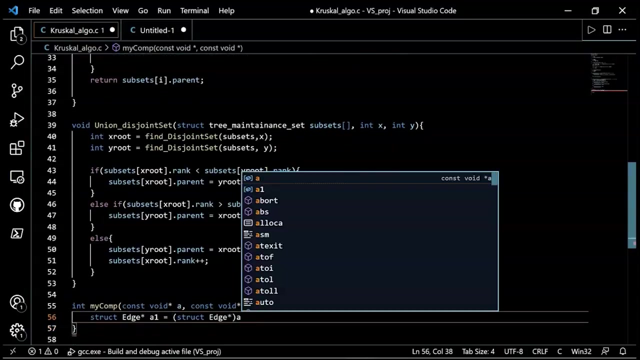 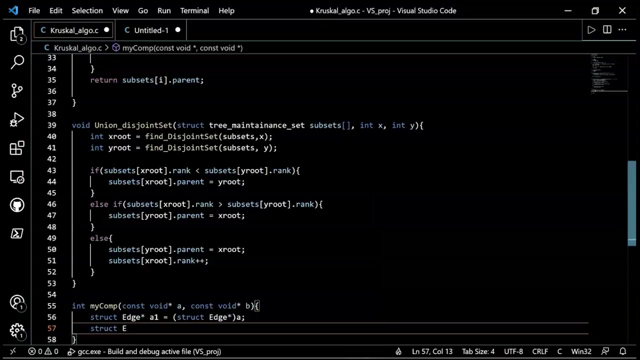 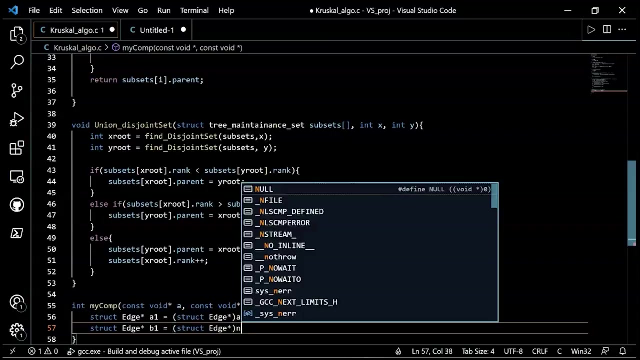 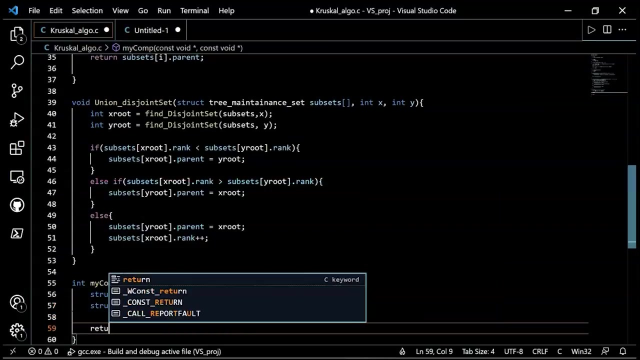 we'll create struct age a. one is equal to struct age φ. ihi a, cyclone 5, three, two. Next, h star b1 will be equal to struct h, star b. Next, we will return the output: a1.weight is greater than b1.weight. 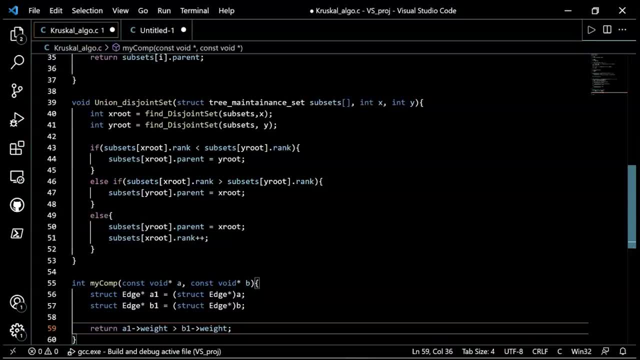 So, basically, what this statement will do is if the weight value of a1 is greater than b1,, then it will return a1 as output, and if the weight value of b1 is greater than a1,, then it will return b1.. 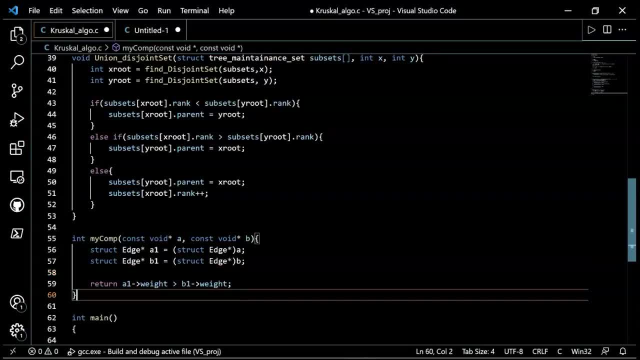 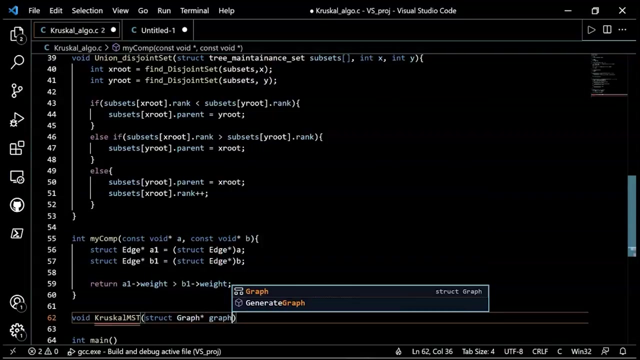 I hope you guys are clear with this- my comparator function. So, moving forward, we will finally create a Kruskal MST function. The return type of this function will be void and we will name this as Kruskal MST And inside it we will pass argument, struct, graph, star graph and we will create function. 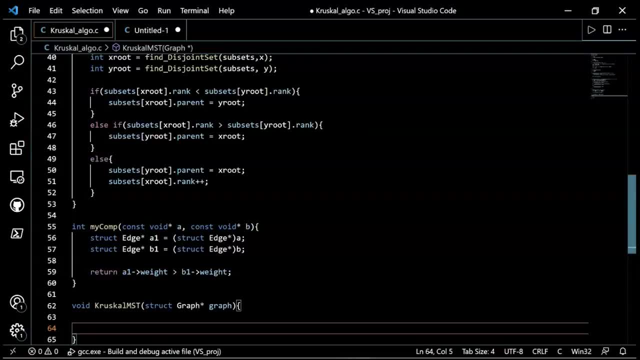 body. Now the first thing that we will do here We will assess the value of number of nodes in a graph and after that we will generate a new reference of structure age for storing our MST. So the first thing we will get the node to graph. dot msd. 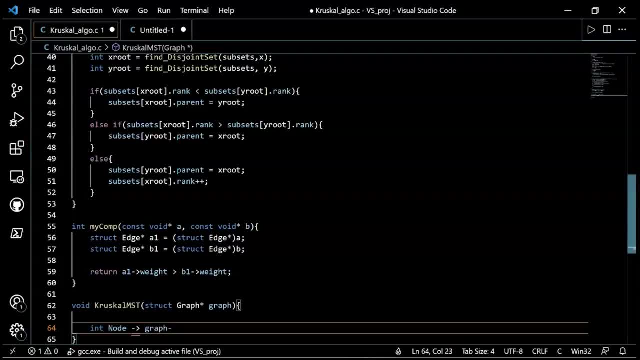 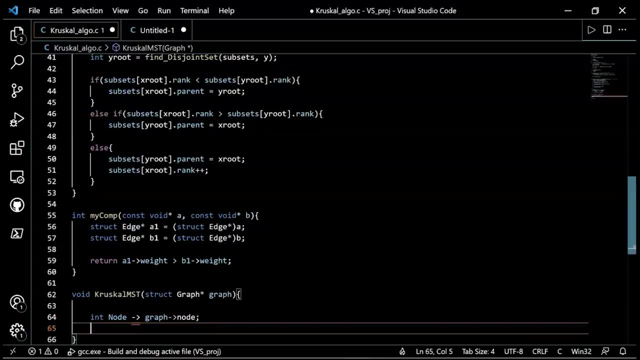 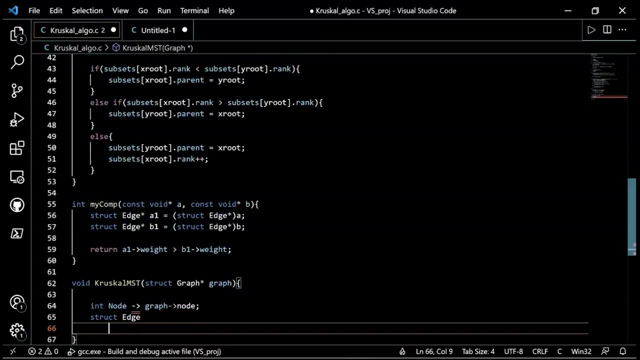 So the first thing we will get the node to graph dot msd. So the first thing we will get the node to graph. So the first thing we will get the node to graph dot msd. So the first thing we will get the result. its set to be no for load, result: your. 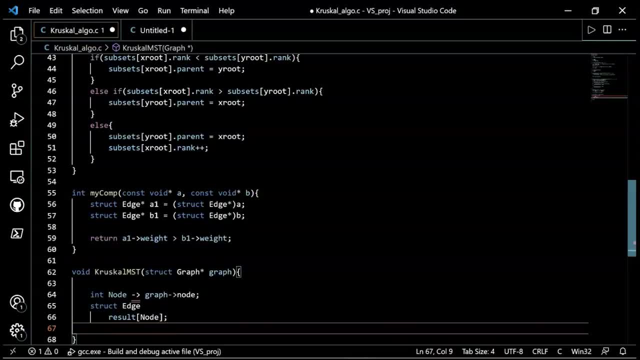 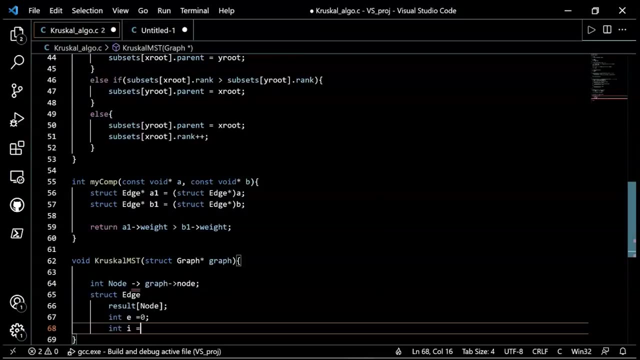 Along with it, we will also initialize variable e and variable I equal to 0.. So that these changes will go. I just happy. So int e is equal to 0 and int i is equal to 0.. We need to break the indentation here and here as well, and semicolon. 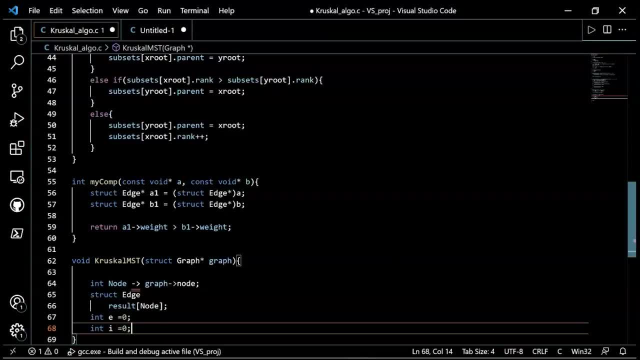 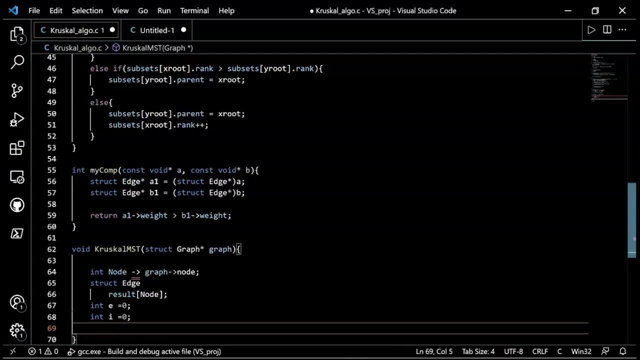 So basically, these variables will store index values for result and index variable for the sorted list simultaneously. Now, moving forward, we'll sort all the edges of a graph. If we are not allowed to change the given graph, then we can create a copy of the given graph. 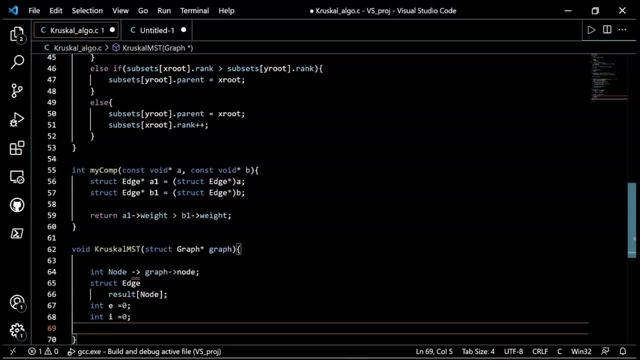 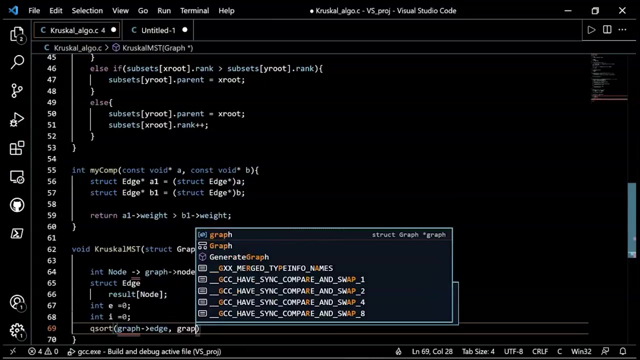 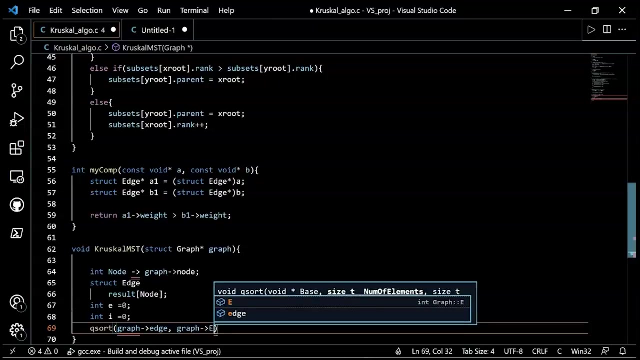 The function named qSort allows us to do that, So let's create that qSort function here. qSort: graph: Edge, comma, graph E, comma. size of graph: Edge, Edge, Edge, Edge, Zero, Zero. 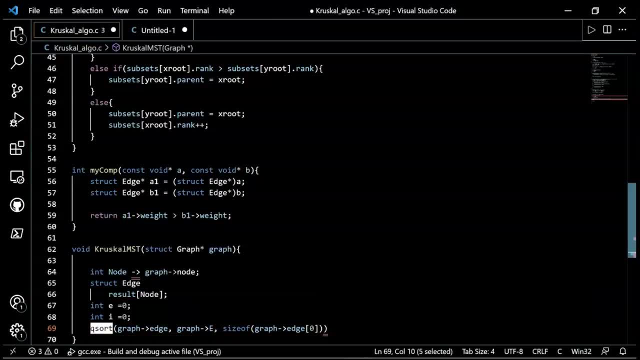 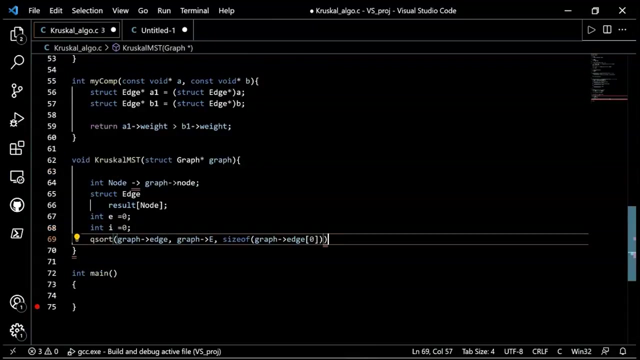 So this qSort is nothing but C standard library function that implements a polymorphic sorting algorithm for arrays of arbitrary objects according to a user provided comparison function. And that comparison function is nothing but this, my comparison function, And I guess You guys must be clear with this qSort term. 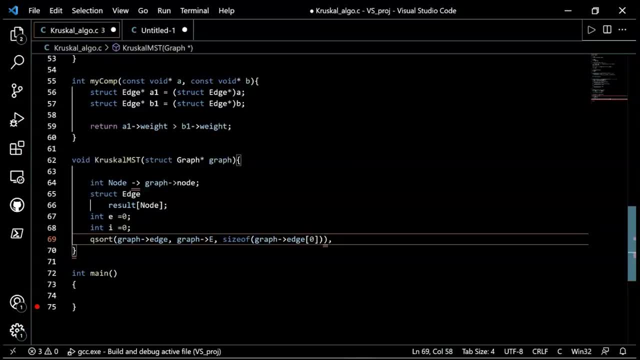 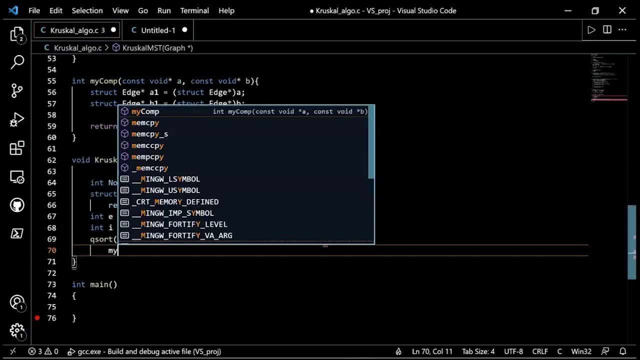 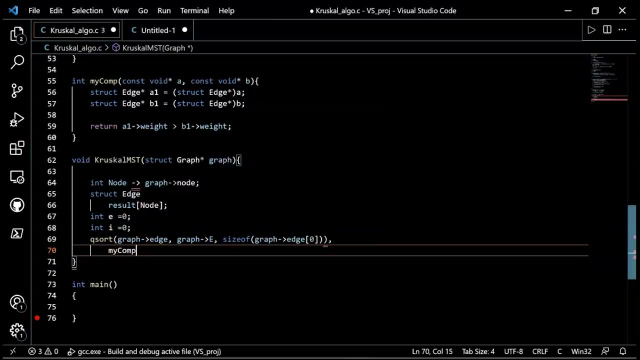 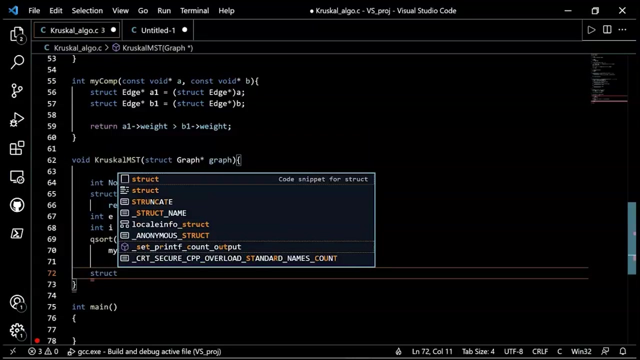 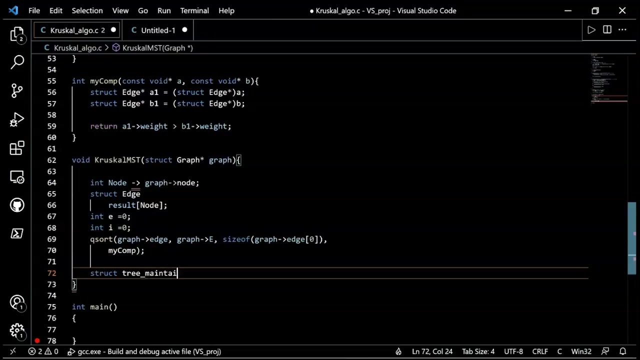 So let's add Comma here and we'll give call to a my comparator function. Now, moving forward, we'll break the indentation and we'll call the object of tree maintenance set underscore maintenance set. star subsets equal to struct. tree underscore maintenance. 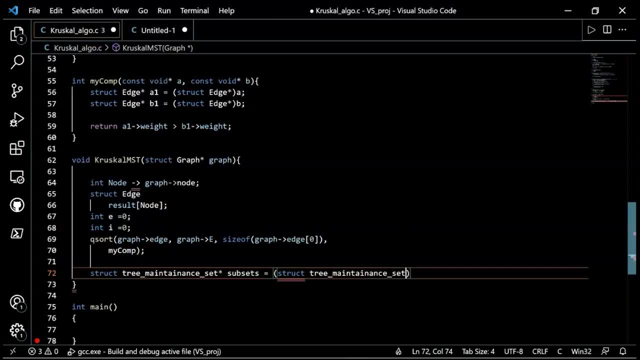 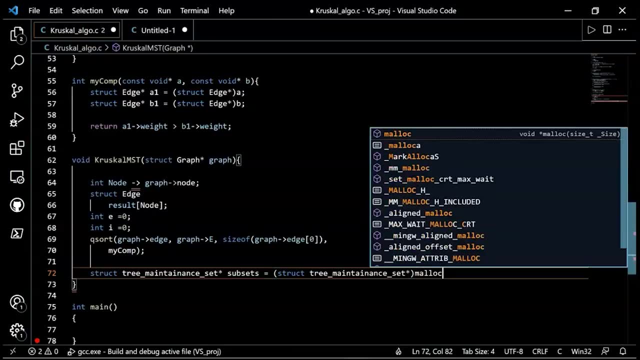 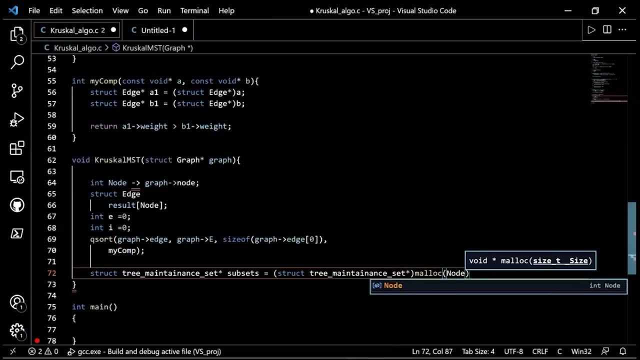 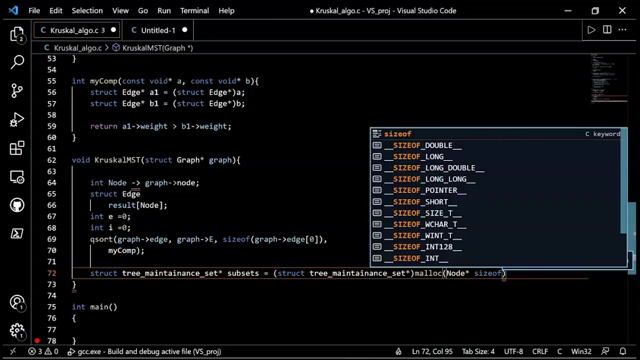 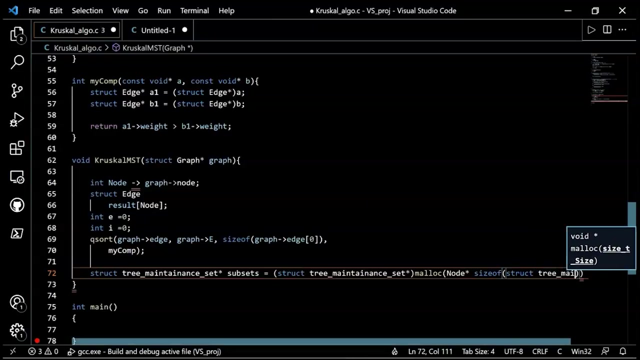 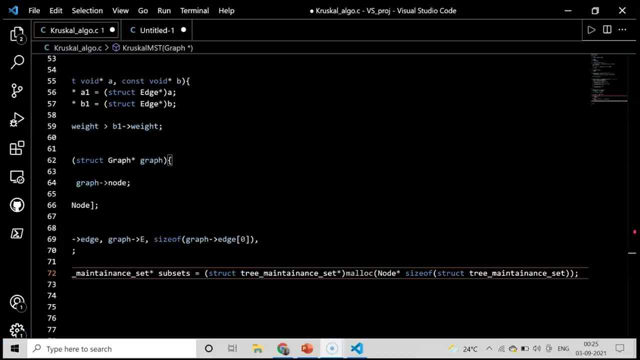 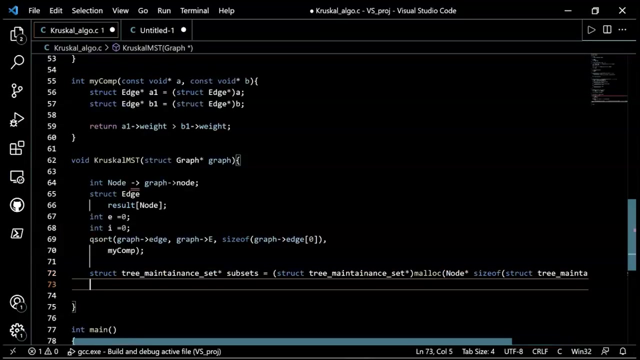 underscore set: star, malloc node, star, size of struct tree underscore maintenance underscore set, and we'll add semicolon here. so next we'll create subsets equal to number of nodes and after that we'll make sure that all the elements have the rank value equal to 0, and to do that we'll initialize new for loop. 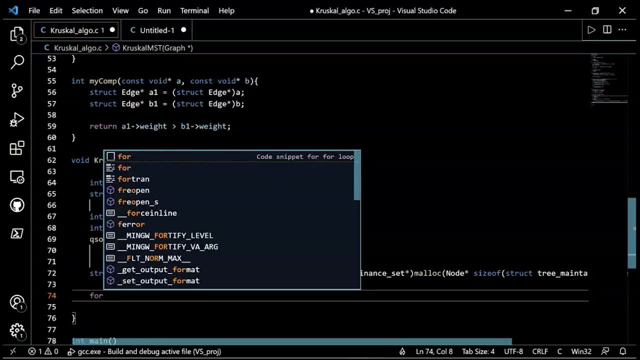 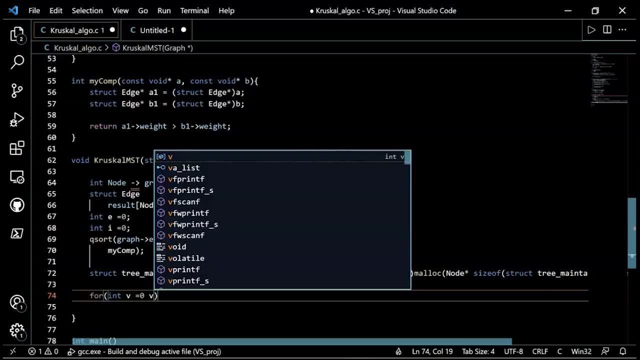 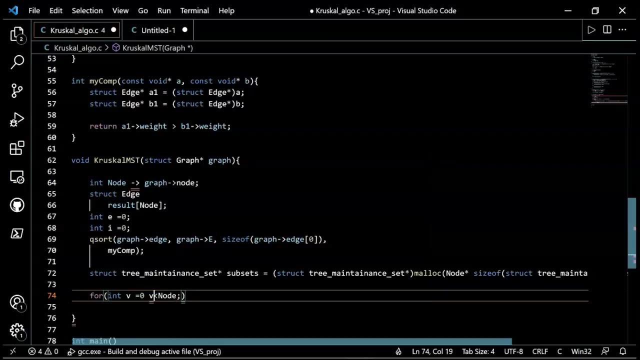 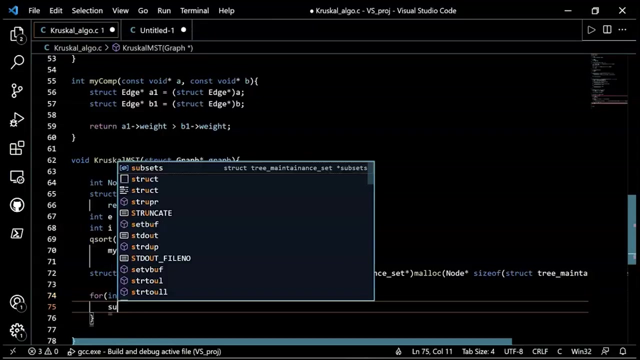 so let's create for loop here. we'll begin it from v is equal to 0 to v- it's less than node- and we'll set this v to incrementation. after that we'll make body for this for loop and inside it we'll set subsets, v. 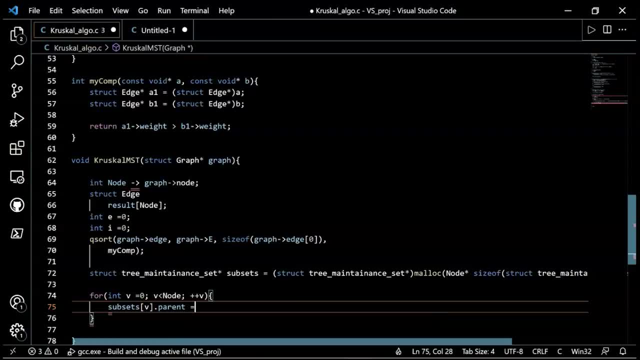 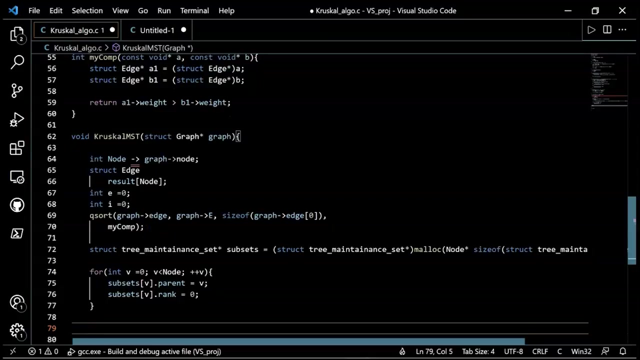 dot parent is equal to v and subsets v dot rank is equal to 0. now, moving further, we'll traverse through all the edges in the graph, but we want to limit our traversal to the number of vertices minus 1, and to achieve that we'll create while loop here, while. 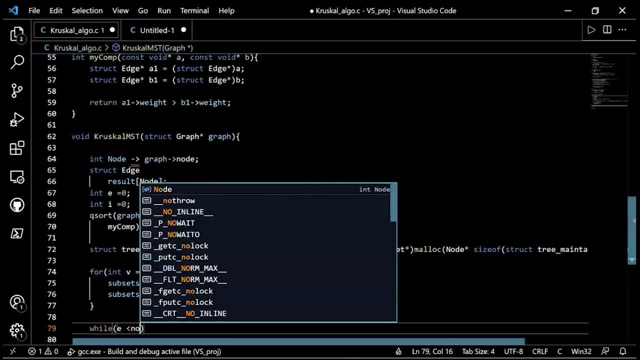 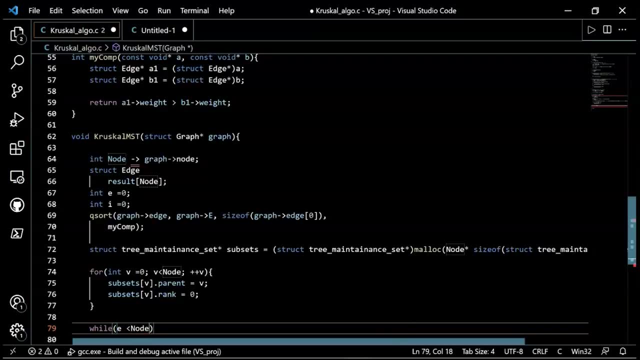 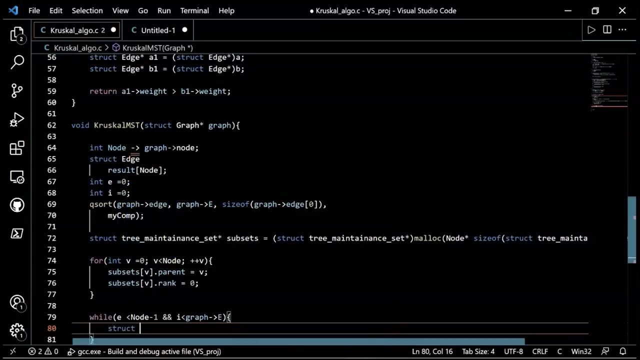 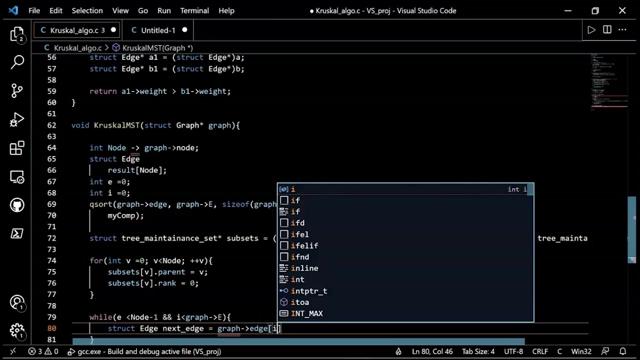 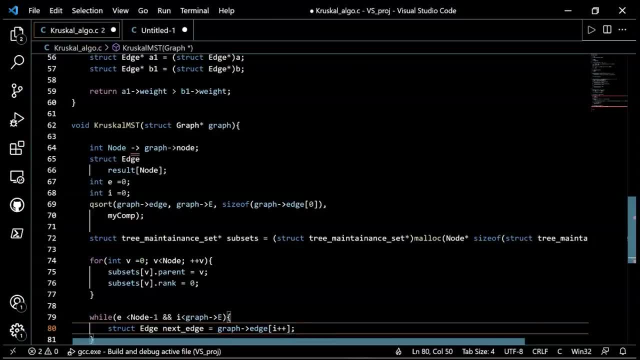 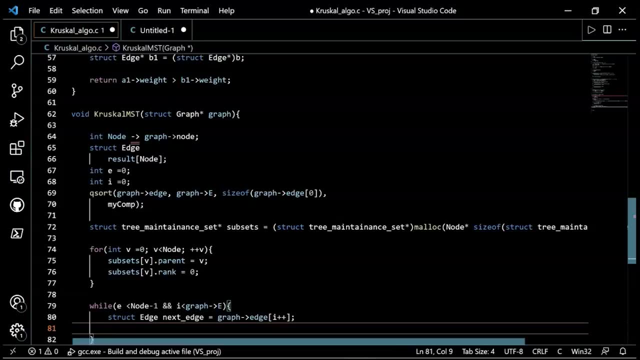 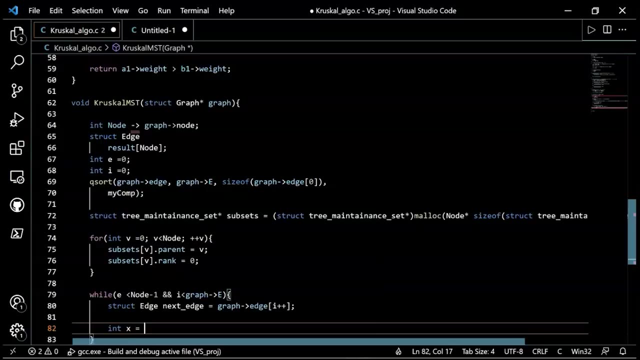 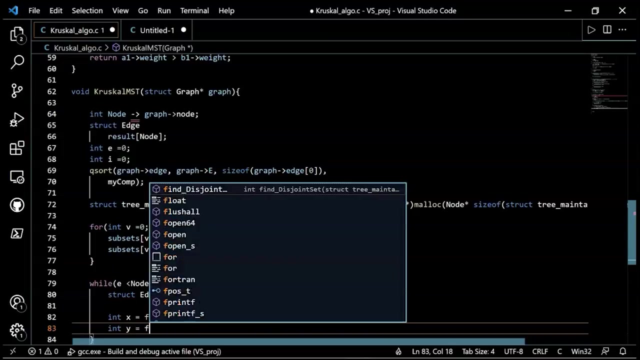 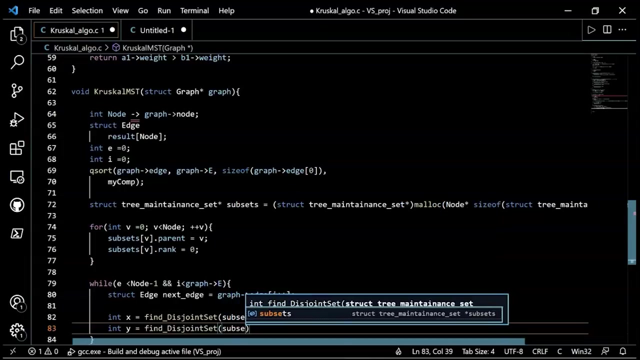 plus, plus in this kinda create X and Y nodes. so let's do that. and X will be equal to find underscore disjoint set and we'll pass subsets comma next age dot source. and for Y will pass find underscore disjoint sets, subsets comma next underscore edge dot destination. 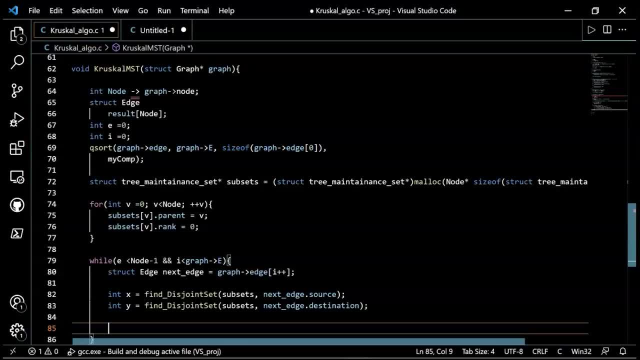 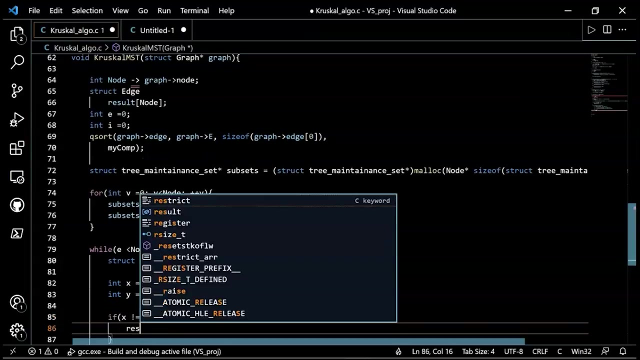 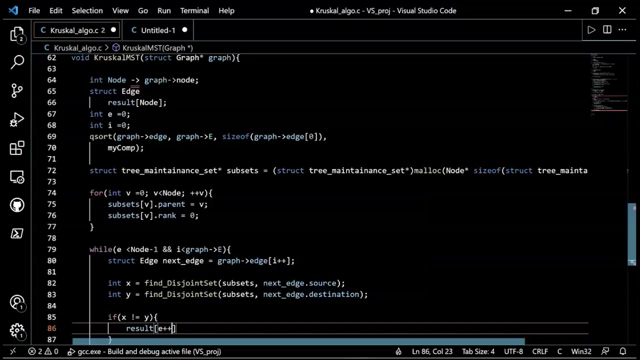 now, if including the age between X and Y does not create the cycle in our graph, only then we can include that edge in our MSD. for that what we can do is will say it's not equal to Y, then we'll set result E plus plus equal to next. 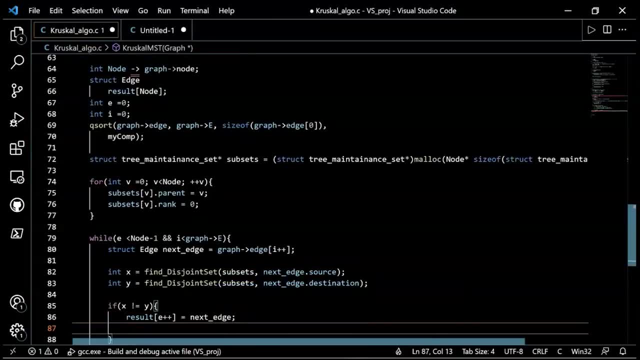 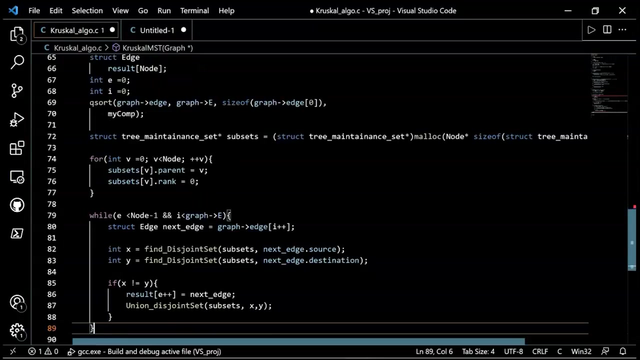 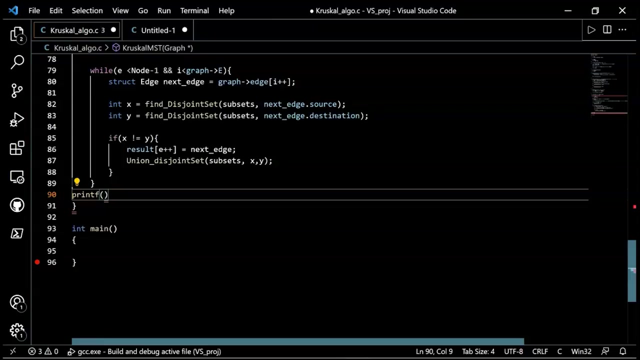 underscore edge and find union disjoint set for subset, and will pass x and y. as with this, we have successfully created our Kruskal's MST function. now what we'll do is we'll also print the structure of our minimum spanning tree. for that we'll need to. 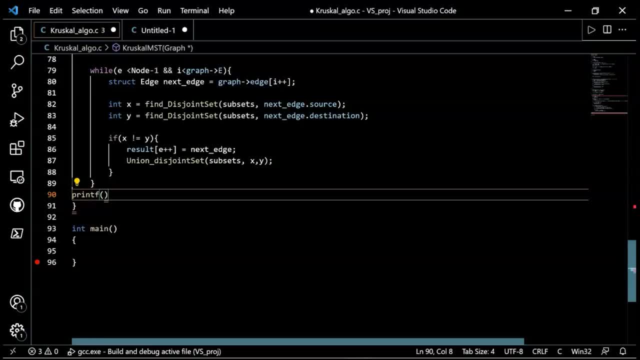 create pattern using printf function. so let's do that. the first statement that will print on screen is: ages created in MST are as below, and we'll add back slash, and so that our Kruskal's MST function will be created in our Kruskal's MST function. so that our Kruskal's MST function will be created in our. 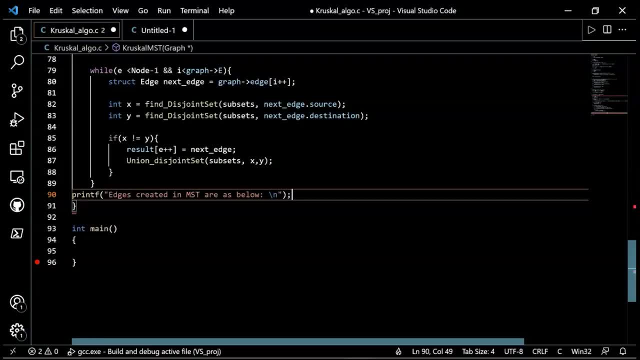 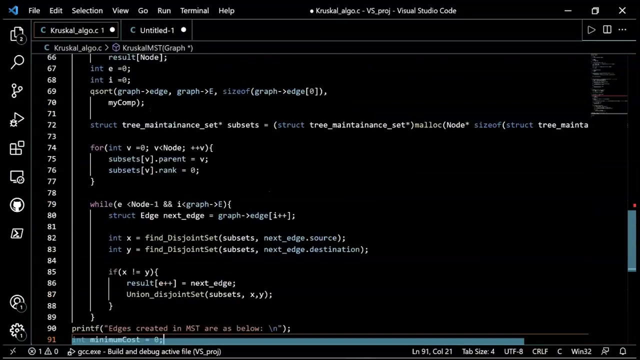 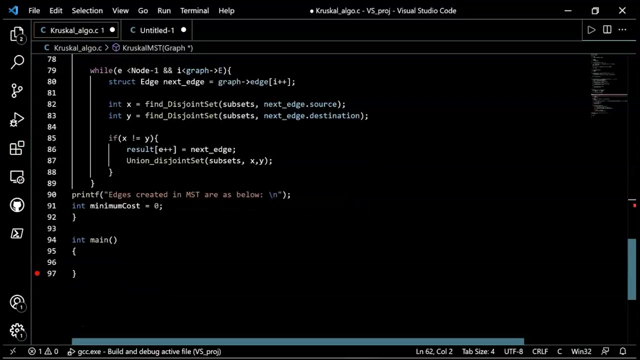 output gets to the next line, we'll add semicolon and that will add end minimum cost variable and will initialize it to zero. okay, so what we'll do is we'll create for loop here and we'll initialize it with I data 11, beginning from 0 till I. 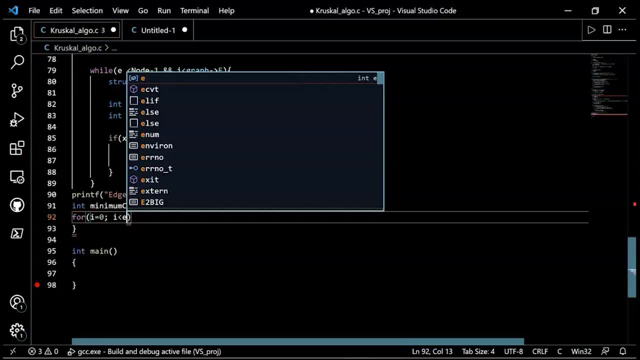 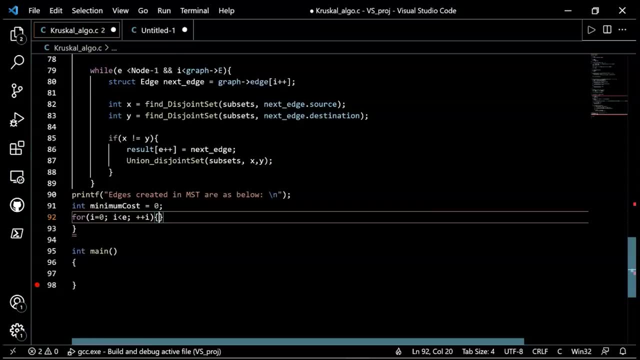 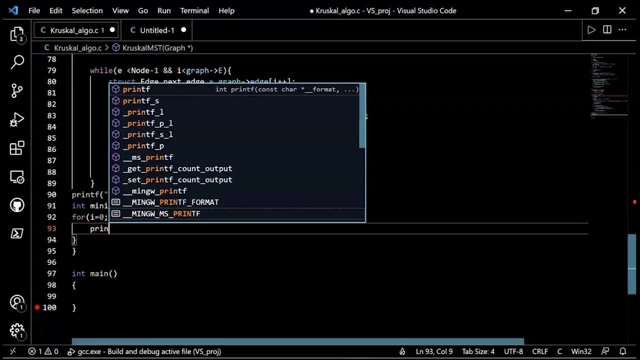 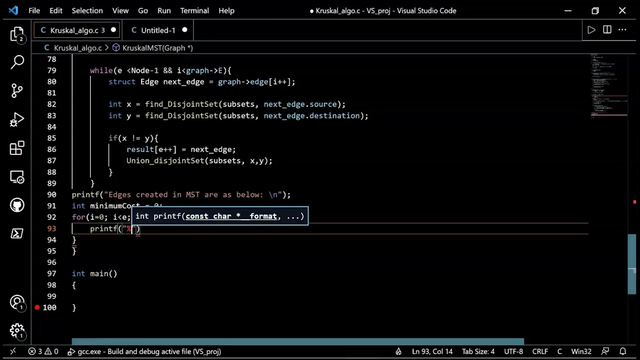 less than equal to e. and when I create this I element, and what will do? it will create pattern for printing the edges. the pattern will go like: modulus D, dash, dash. modulus D equal to equal to modulus D, slash, and. and the parameters that will get printed will be: result: I dot source. 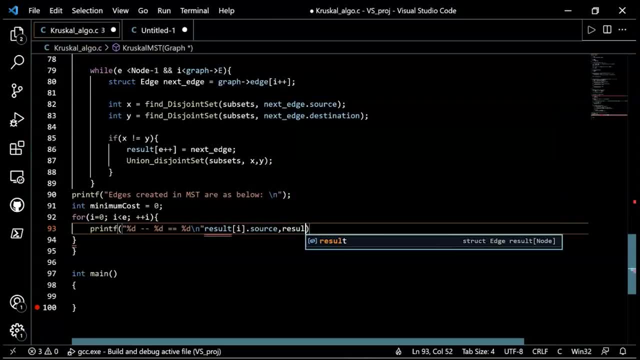 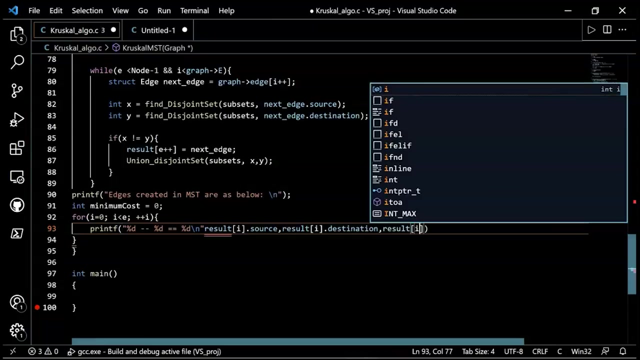 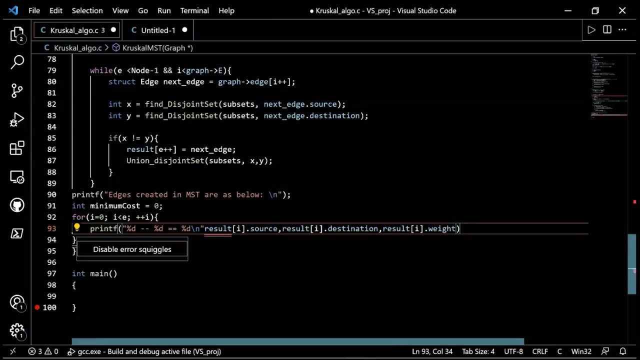 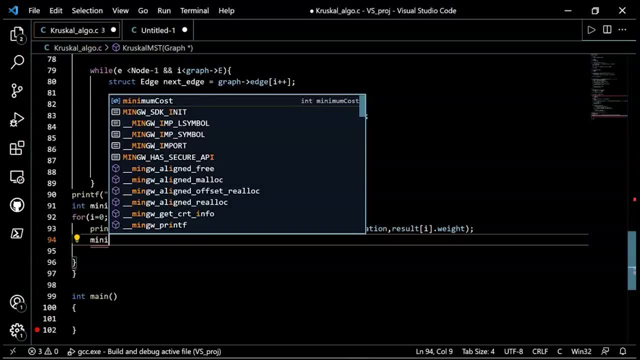 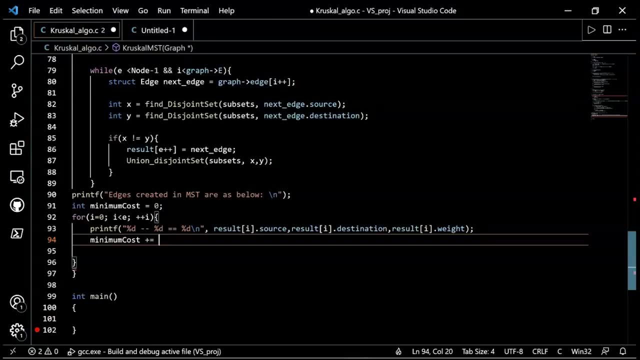 values of edges to it. so we'll take this minimum cost variable and we'll add the result. I dot wait to it. now. we'll get outside this for loop and we'll print F. one more statement: the cost for creating MST is modulus D and we'll print minimum cost KV. 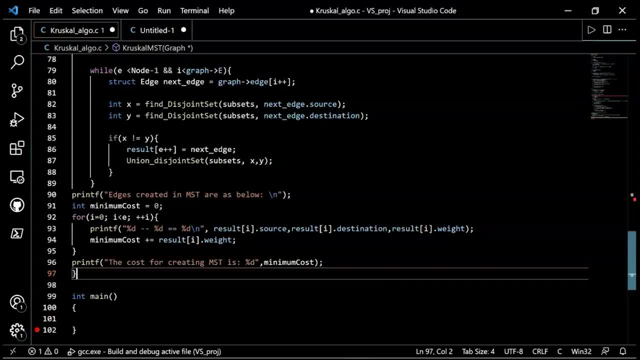 that is less than average. so we have now successfully implemented Pascal algorithm function, and we have created code for printing it on console as well. so now, moving forward, we'll work on our driver method, and for that let's get into its function. body here first will define the number of nodes that we 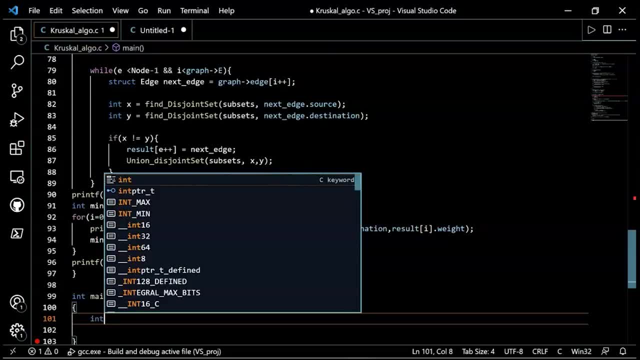 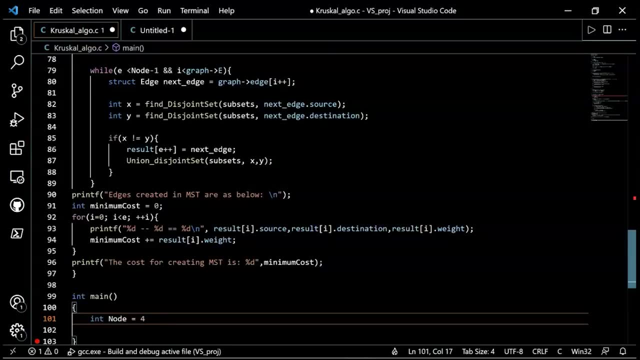 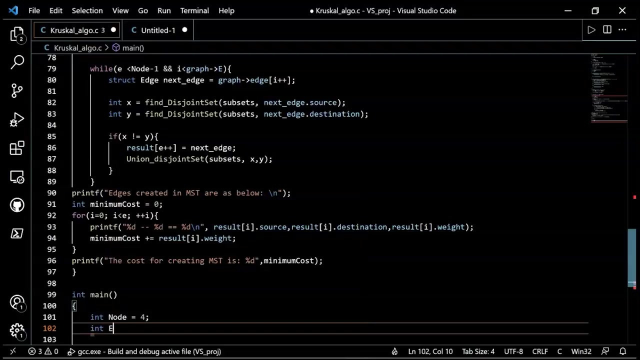 are going to use for a graph. number of nodes are four. the graph structure that we are going to pass to this Kruskal's algorithm program is the same that we have discussed implementation strategy, for. it had four edges and it also had six edges as well, so we'll add six edges here. 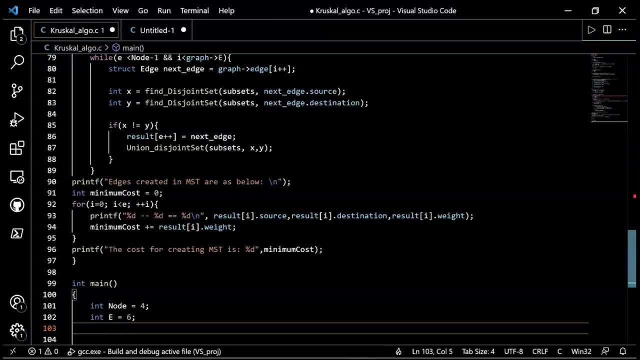 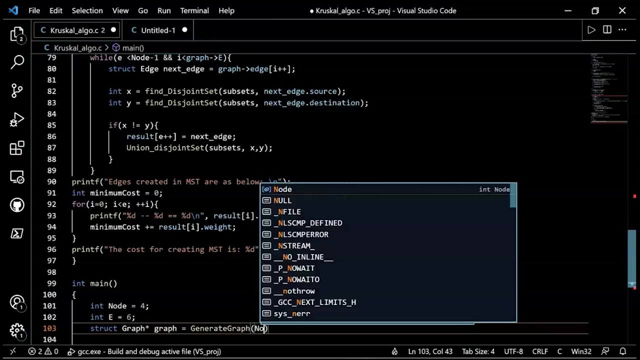 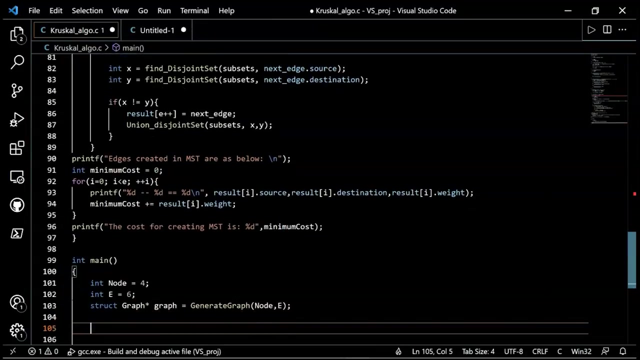 now what we'll do is we'll set struct graph, star graph equal to generate, generate graph, and we'll pass node comma e and we'll add semicolon now. next, we'll create graph structure by implementing the edges, so the for first edge will call graph dot edge, zero dot source. 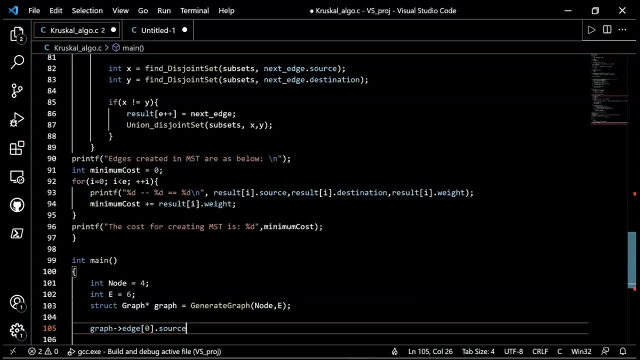 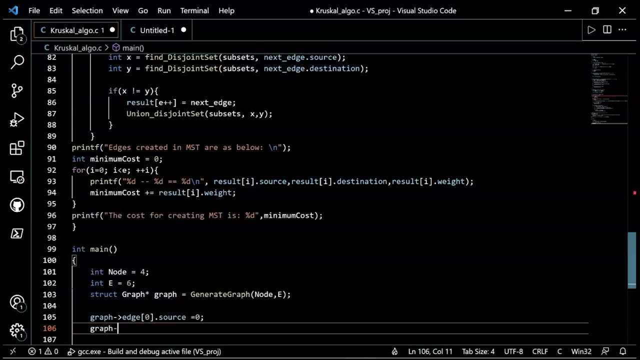 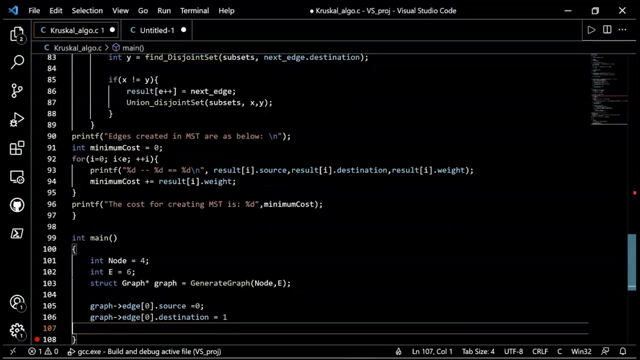 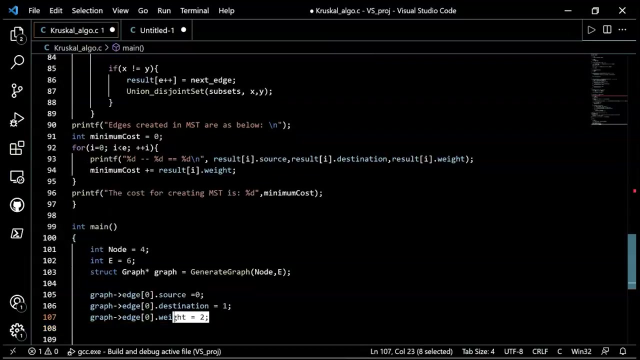 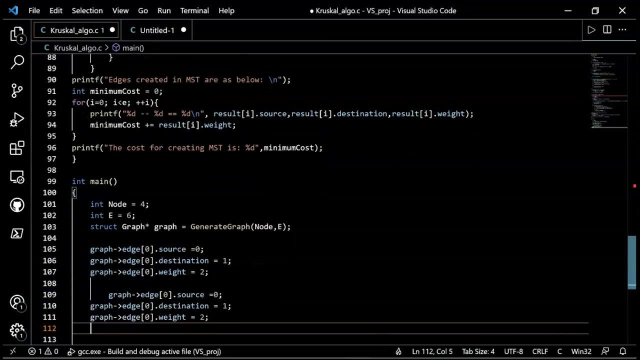 zero dot source. zero dot source will be equal to zero. that means the first edge will begin from zero and it will end at destination node, and that will be one, and the weight for this age will be equal to now. we'll copy this pattern and we'll paste it below. okay, and now the age will be one. 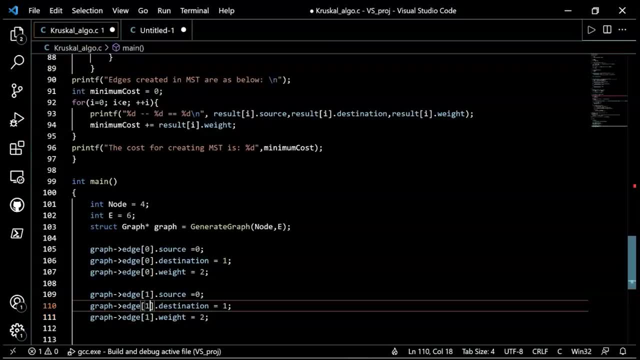 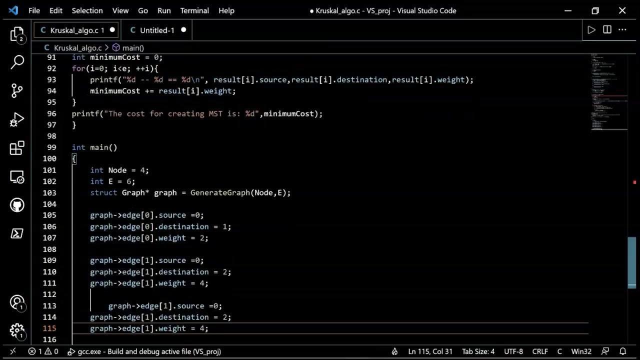 and for this age one, the source will be zero and destination will be two and the weight value will be four. now let's copy this again, paste it and we'll set age number to two. will change source and destination. now, source will remain same and destination will be changed, will make it three and the weight value will. 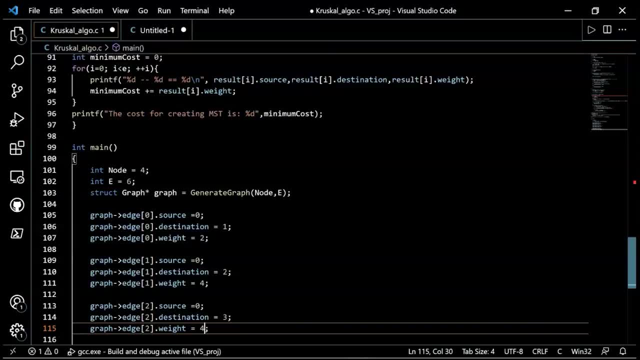 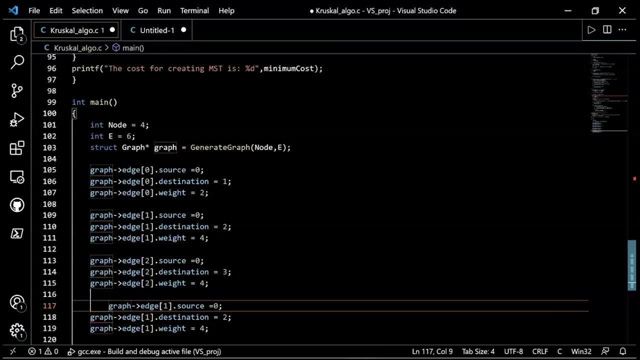 also remain the same. that means age between zero to two and age between zero to three have same age value. press ctrl and wait now for next control. V will remove this indentation. and now we'll change the node number, edge number. here the swims will be one and destination will be. 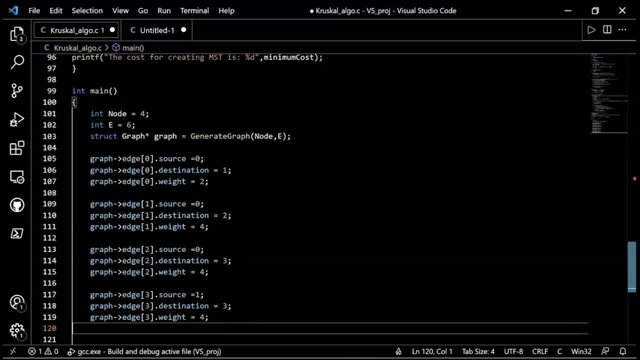 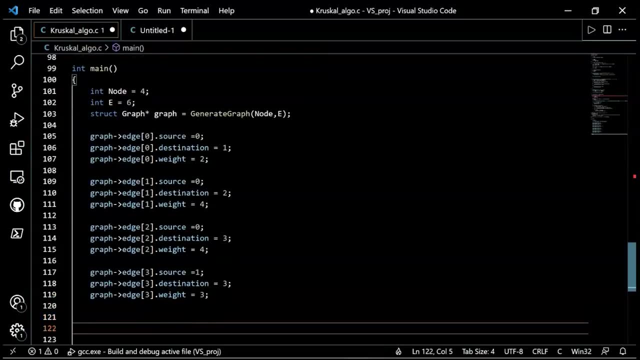 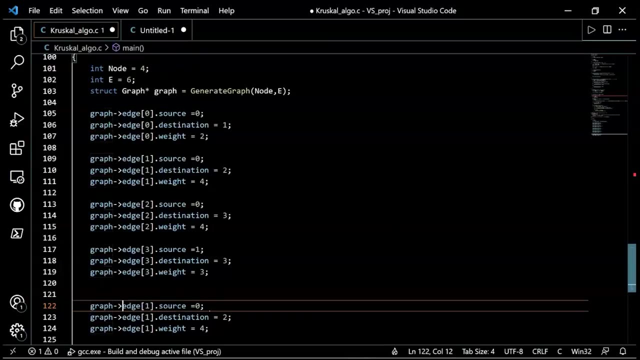 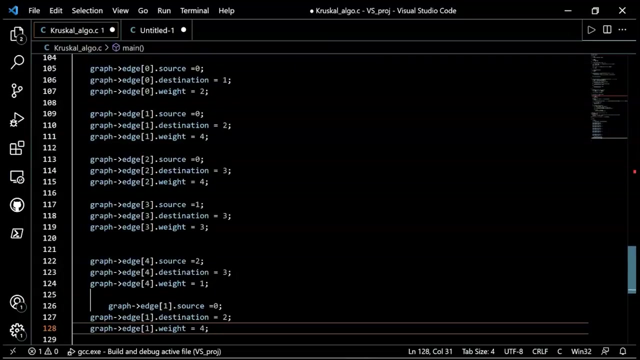 three And the age-weight value will be 3.. After this, we'll add new age. The age number will be 4 now, The source will be 2 and destination will be 3 and age-weight will be 1.. And the last age will be age 5.. 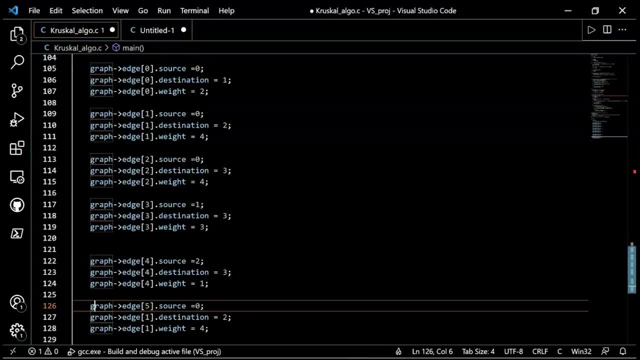 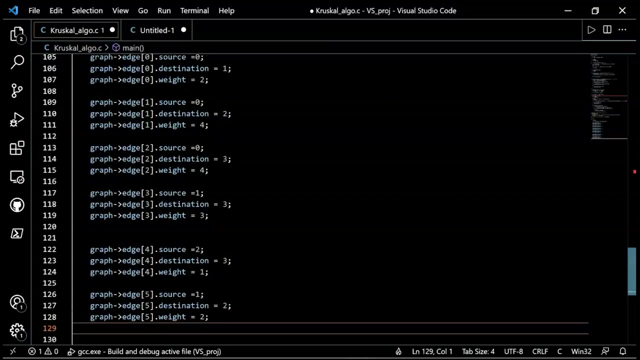 And the last age will be age 6.. And the source will be 1 here, and destination will be 2.. The age-weight will be 2.. Now, after this, what we'll do is we'll give call to our QsqlMST function. 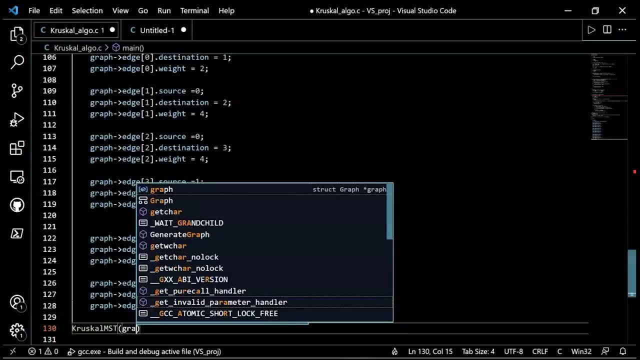 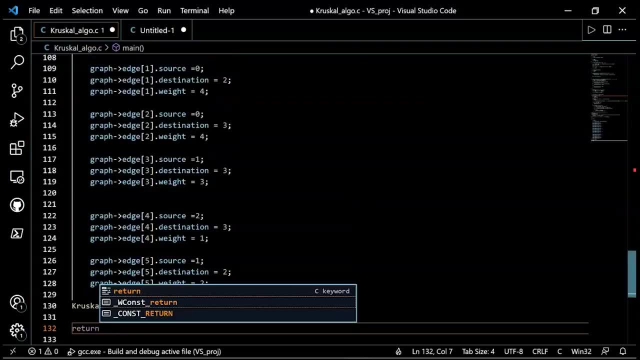 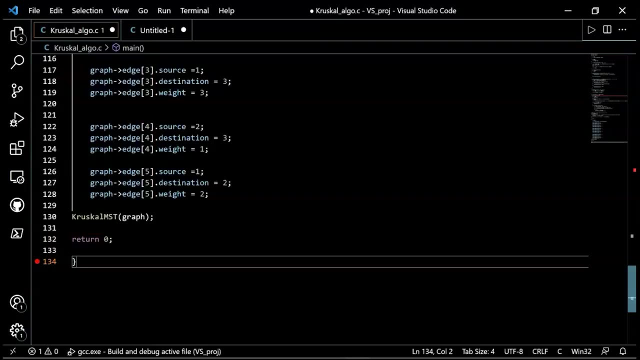 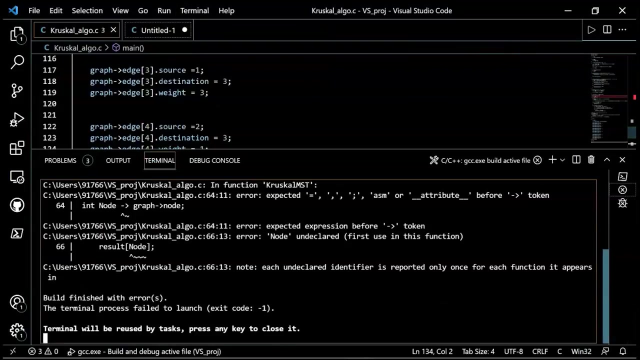 In order to generate minimum spanning tree, and we'll pass this graph structure to it And we'll add return 0 statement. With this, we have successfully completed our programming implementation for Qsql's algorithm, So let's run it and check if our code is working fine or not. 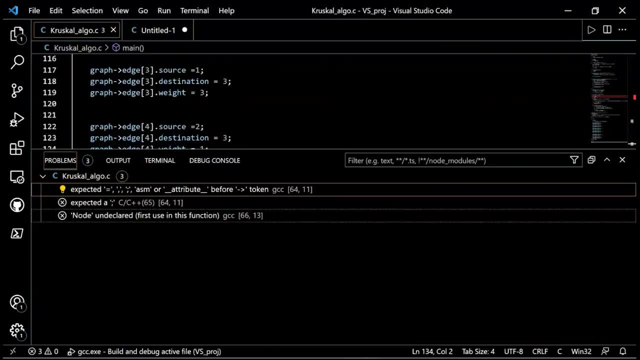 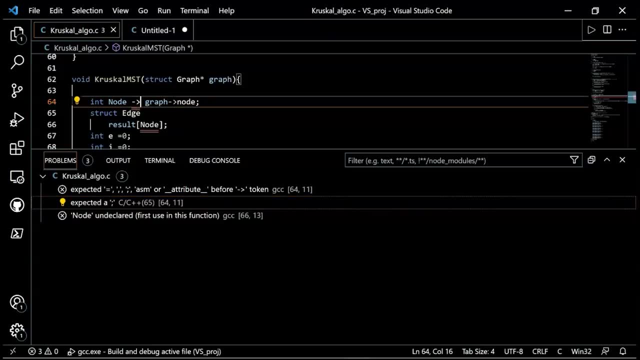 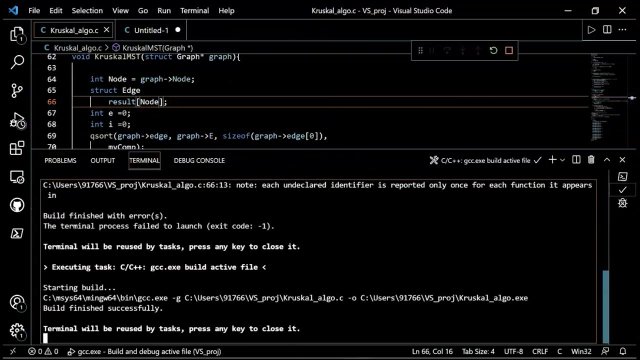 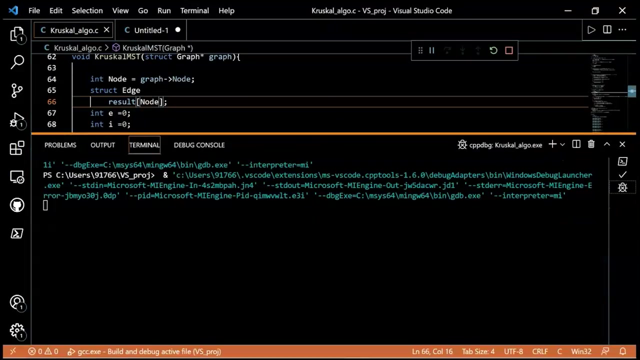 Okay, so we are getting three problems here. The first one is expected token, So int node will be equal to graphnode, And this node should also be capital here. Okay, So what next error is there? Yeah, So now our code is bug free.